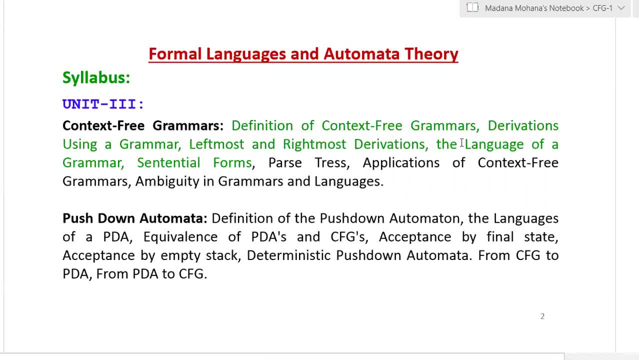 derivations, that is the leftmost and rightmost derivation, then language of a grammar sentence, waveforms. So all these topics we will cover in this lecture. Next lecture we will continue with remaining topics like parse trees, applications of context-free grammars. 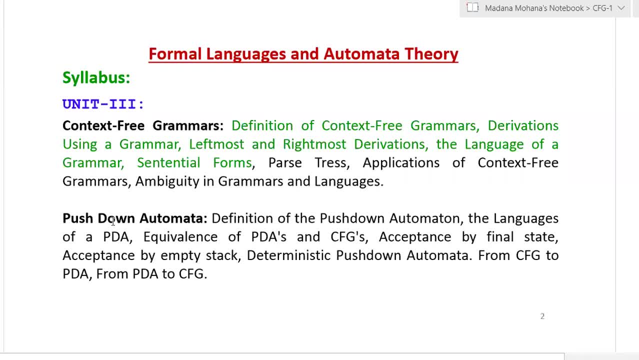 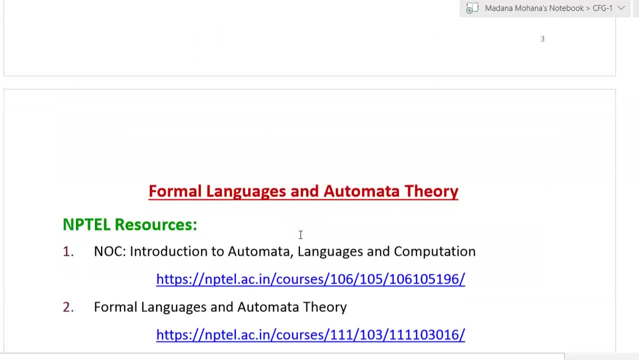 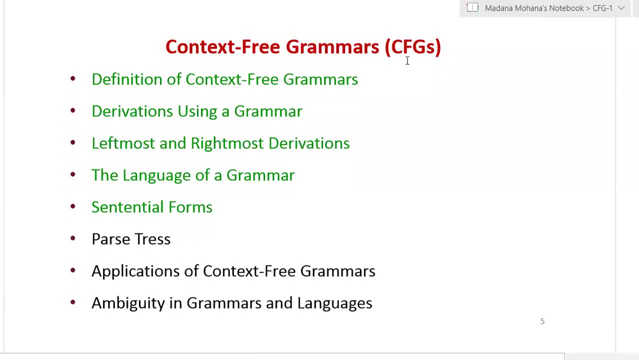 ambiguity in grammars and languages. Later we will discuss about its acceptor, that is, a pushdown automata. Now let us see the outline or agenda of today's lecture. Introduction to context-free grammars. First we will see the definition of a context-free grammar. then, what is a definition? 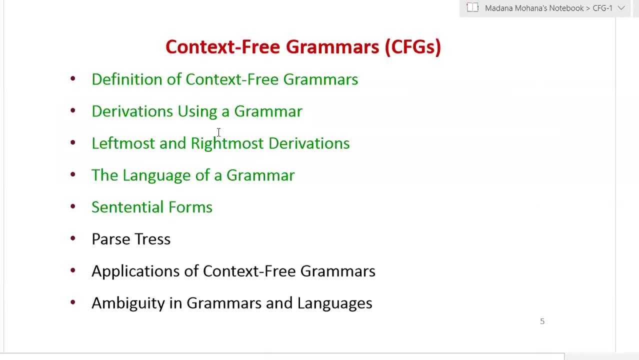 derivation: how to define a derivation using context-free grammar. then types of derivations. There are two types of derivations: leftmost and rightmost derivations. Then how to find long ways of a context-free grammar. Then, what is a sentential form? What are various? 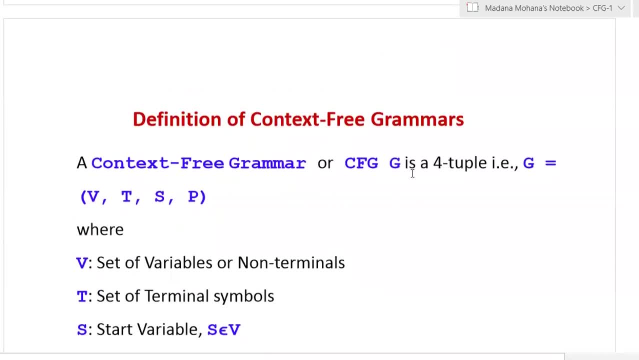 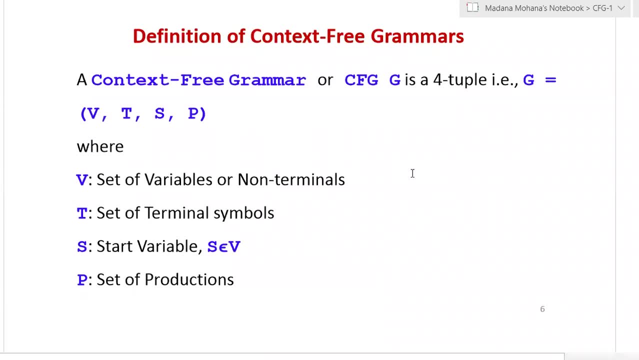 types of sentential forms. So these topics we are going to cover here. Now let us see definition of context-free grammar. We already know the definition of a grammar: a formal grammar or a grammar which is defined as a portable. that is, G equal to VTSV, So any 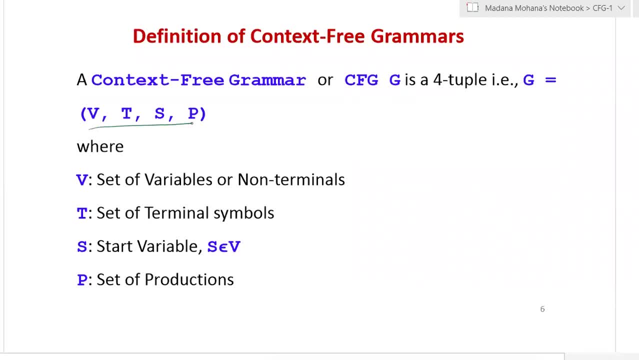 grammar. the formal definition is same. The only difference is grammar to grammar. only the production rules are changed, So remaining all tuples are same. Here also a context-free grammar, also abbreviated as CFG, denoted by G, is a portable, that is G equal to VTSV. Except production rules, all tuples are same. 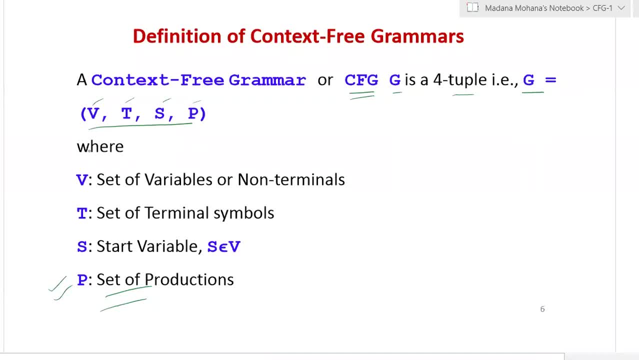 as in formal grammar or regular grammar, where V is set of variables, also called as non-terminals, whereas T is set of terminal symbols, Whereas ST is the start variable which belongs to the variable V, where P is set of productions. 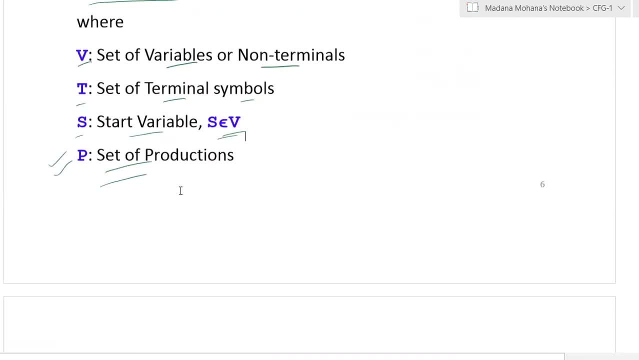 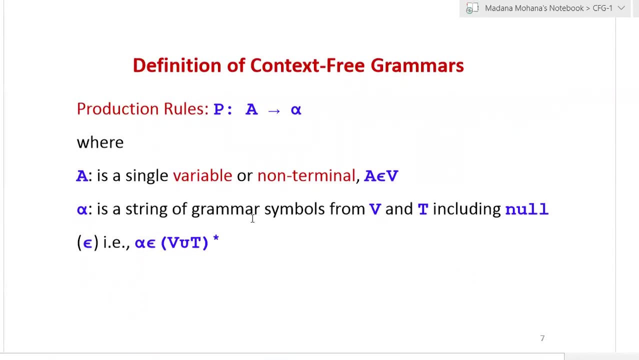 So all tuples are same. Now let us see the rules of productions in context-free grammar. What are the rules? The production rules are of the form a derives alpha, Production's a to alpha. where left hand side of the arrow you can see we have only one variable. that is capital. 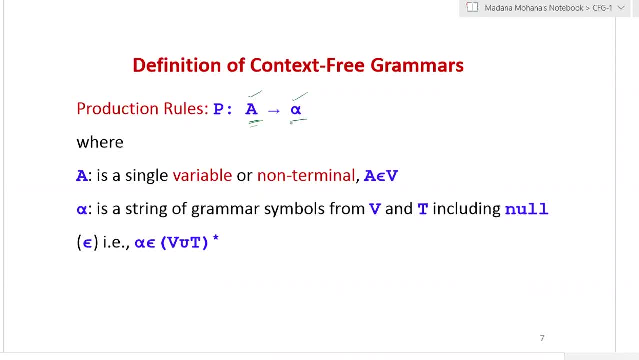 a, whereas right hand side of the arrow we have alpha. now, what is a? what is alpha here? c, where a is a single variable, or non-terminal, where a belongs to the set v variable, set of variables. so, left hand side of any context, free grammar- it contains only a single variable. that is the. 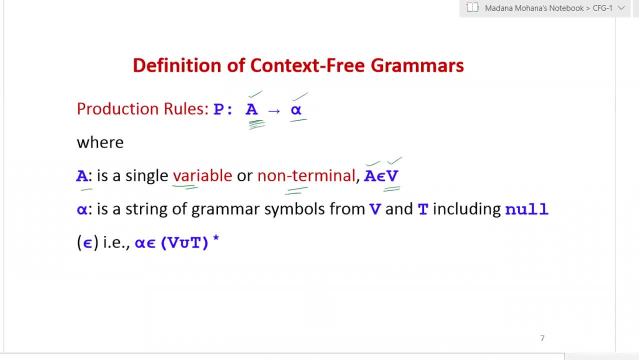 restriction, whereas alpha the right hand side of the production. alpha is a string of grammar symbols from variables and terminals which includes null also, that is epsilon or lambda. that is defined as alpha belongs to v, union, t, whole closer, that is star, closer means which, which includes null also. so in normal definition of a formal grammar, alpha is same. 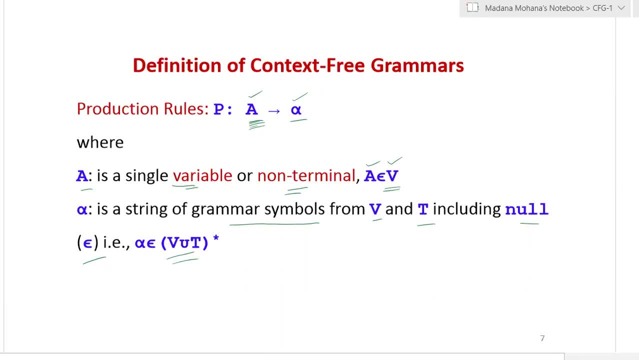 i mean right hand side is same, that is v unity whole closer, whereas left hand side in normal grammar we have taken v union t positive closer, v union t positive closer. so left hand side it does not includes null. this is normal grammar production rules, but whereas in context free, 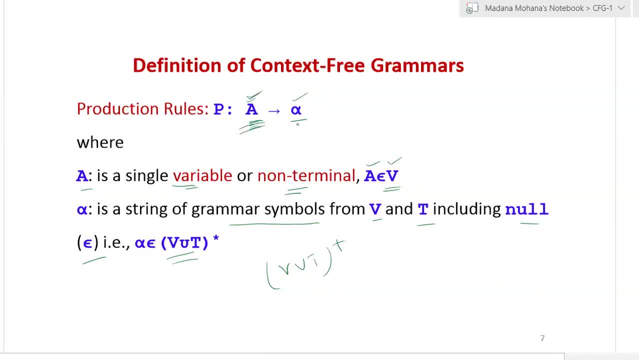 grammar left hand side contains a single variable. right hand side variable or terminal or combination of variable terminals including null. so that is the difference between normal grammar and this context, free grammar. again you can see regular grammar also. you can recall once regular grammar, so regular grammar productions are so: a derives b, c or a derives c. see left hand side also. it. 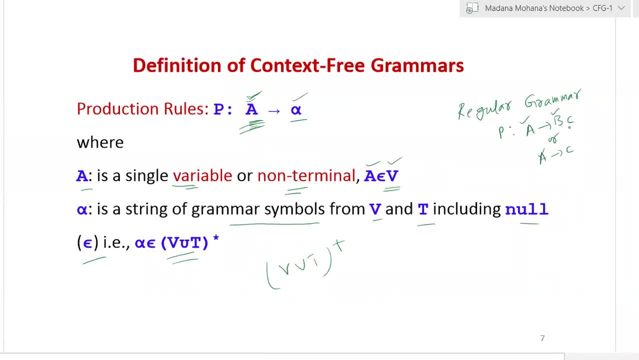 contains single variable, right hand side, a variable followed by a terminal or a single terminal. so this can also be written as a derives terminal followed by variable. so based on this, we can say right linear grammar, left linear grammar, so whereas context free grammar, there is no restriction in the right hand side. 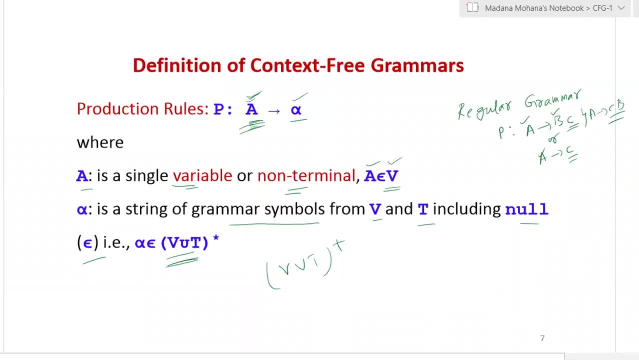 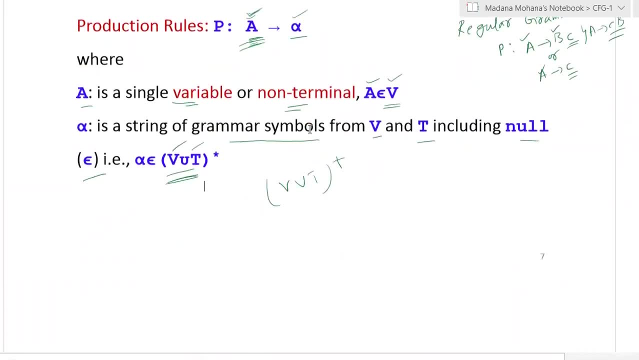 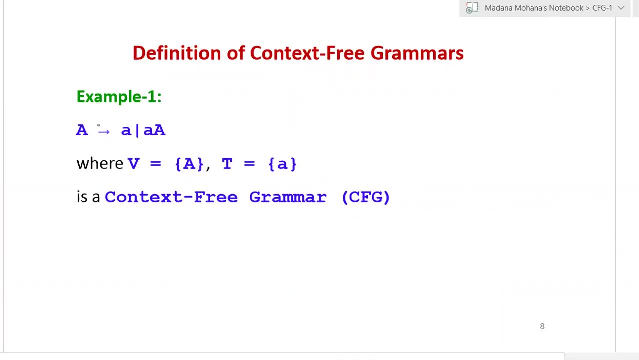 right hand side, it contains any string of symbols from variables and terminals, including null. but left hand side, same restriction as in regular grammar. now let us see some examples. first example one. so the production is like this: a derives terminal a or terminal a followed by variable a. so in this production you can define: 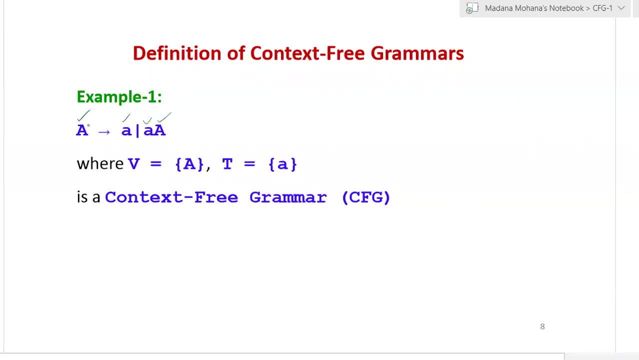 where v variables, variables are only one variable, uppercase letter, so a then terminals are: we have only one single terminal that is lowercase letter, a small a. now it is a context free grammar. how can you say it is a context free grammar? as for context free grammar condition, left hand side, it contains a single variable. it satisfies right hand side either. 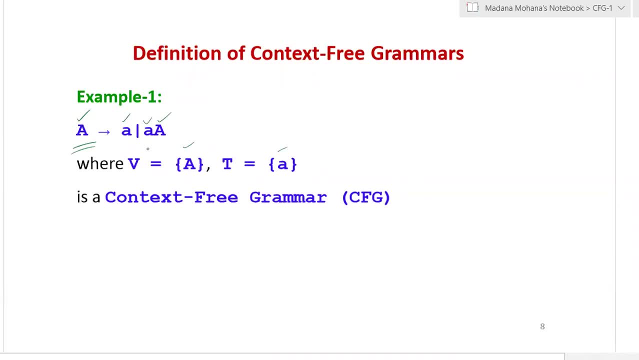 a string of terminals with terminals and variables. so here we have a single terminal, here terminal, followed by variable, including null also, but here null is not there. so so v union t, whole closure. any condition is satisfied, either a variable or a terminal, or string of variables and terminals including null, but it satisfies the condition of a single. 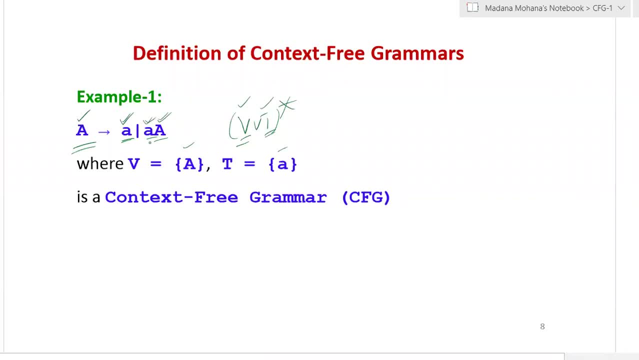 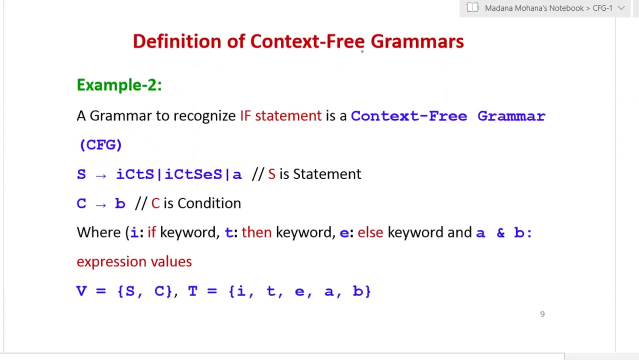 terminal is the terminal, followed by variable. so this is string, string of terminals and variables. so this production satisfies the rules of context free grammar. therefore this is a context free grammar. let us see another example: a grammar to recognize if statement in our computer programming languages. how to define if condition, so that can be described by using context free grammar also. so the definition is: first, s derives i c t s or i c t s e s or a, where s is nothing but statement. so now, in the rest, that's a UI, gluten colocar mixed, which is null. 2 for r, that's a. 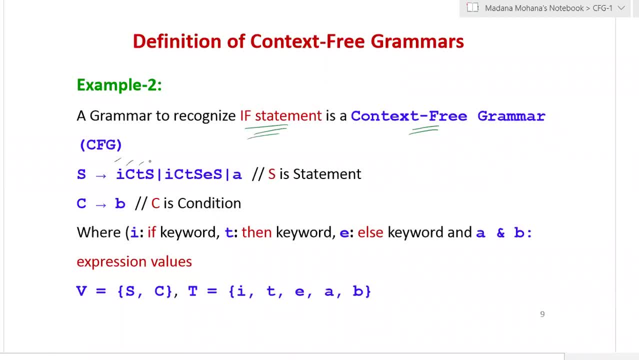 first s derives i c t s or i c t s e s, r a, Ei, ei, where yes is nothing but statement. so now in the rest, that's. or i c t s e s, or a, where s is nothing but statement. so now in the right hand side you can. 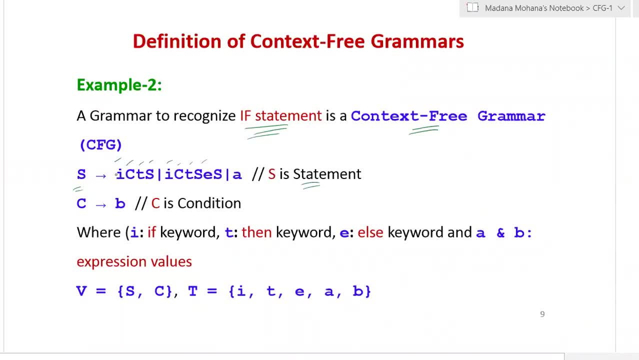 see. so what we have: small i, small i is if keyword, then small t is then keyword, then small e is else keyword and small a, small b are expression values. now here c derives b, where c is a condition. so b is expression value now in our programming languages if condition. how to define if? 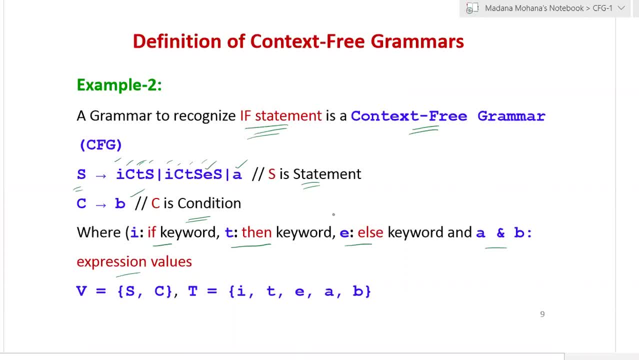 condition, then statement, else condition, then statement, true part and false part. we have two parts. so same thing can be represented using context-free grammar, you using this definition. now, in this grammar the variables are all uppercase letters. we have capital s, capital c, here also capital c. therefore variables are s and c. now terminals are all. 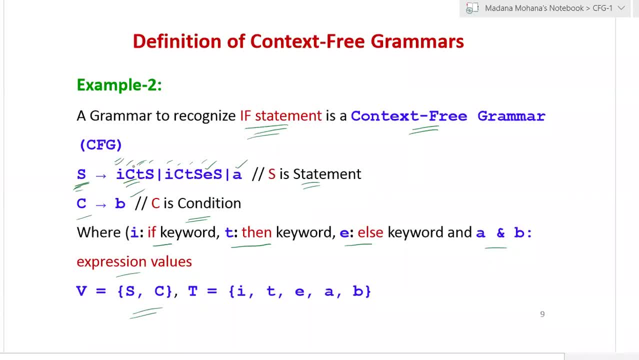 lowercase letters. what are the lowercase letters? small i, small t, small e, small a, small b. so these are all called as terminals. so check whether this is a context-free grammar or not. left hand side: you can see it has a single variable. so any variable, but it contains only. 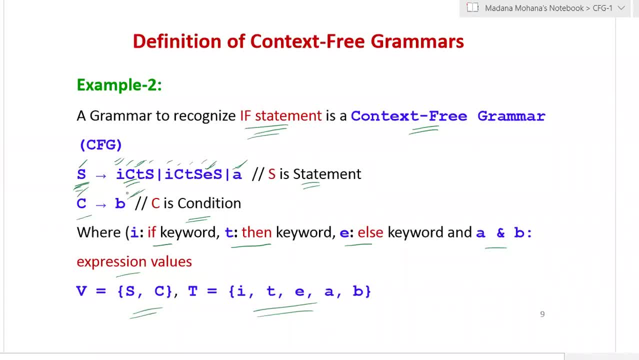 single variable, any value of the variable right hand side, either a single terminal or a single variable or string of variables and terminals- here c, i, c, t, s, terminal variable, terminal variable, string of terminals and variables. here also terminal variable, terminal variable, terminal variables. so even sometimes null also allowed. so therefore, this product, all this production, 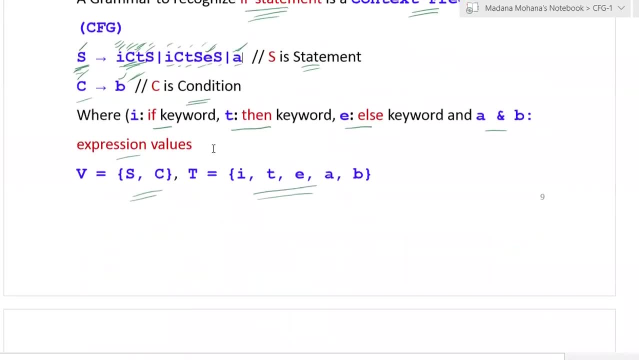 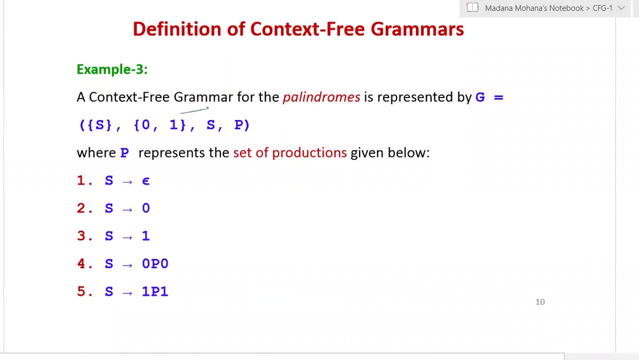 satisfying the conditions of contextual grammars. so this is a context-free grammer. now let us see another example: palindromes string. a context-free grammar for palindromes is represented by g equal to. here. the first set is called as variable v. that is very true. 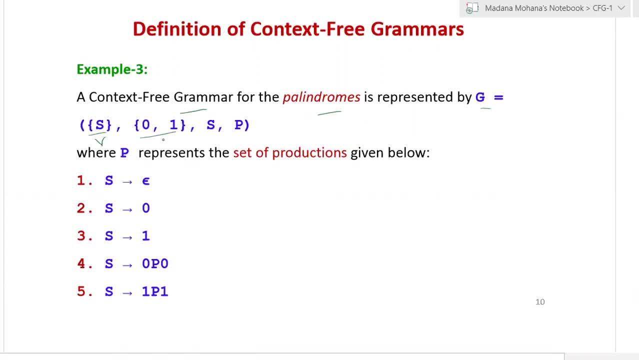 um, it's very awesome and really reporters are really very interested in this particular. that is yes. then second set is called as t, now t, equal to 0, comma 1, then s, p, so v, t, s, p, the order we have to follow. so here variables are yes, only s is given, terminals are 0, 1. 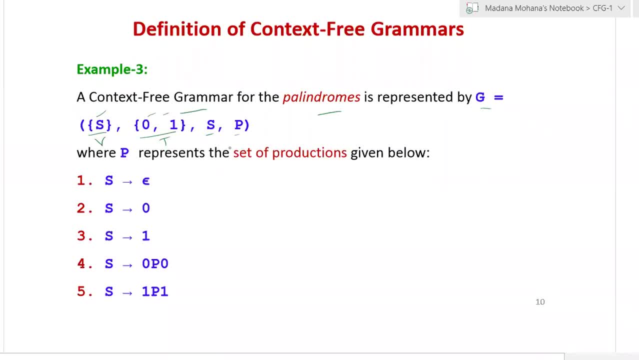 starting variable is s itself. now productions, where p represents set of productions, are given below. the first production s derives null, epsilon or lambda. second production s derives terminal 0. here, 0 is the digit, which is a terminal. now, third production s derives 1. this is also a digit. 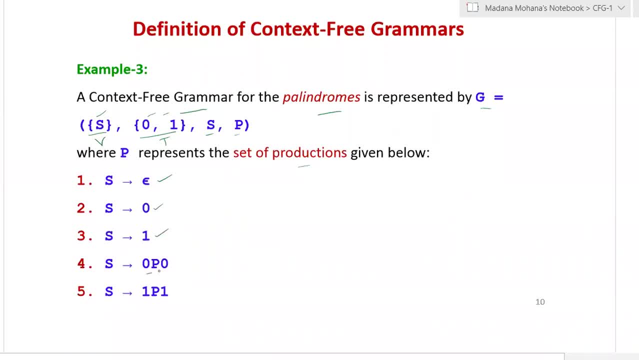 so which is a terminal? now for the production s derives 0 p 0. here 0 is terminal, p is variable, again 0 is terminal. next, production s derives 1 p 1. so 1 is terminal, p is variable, then 1 is again. 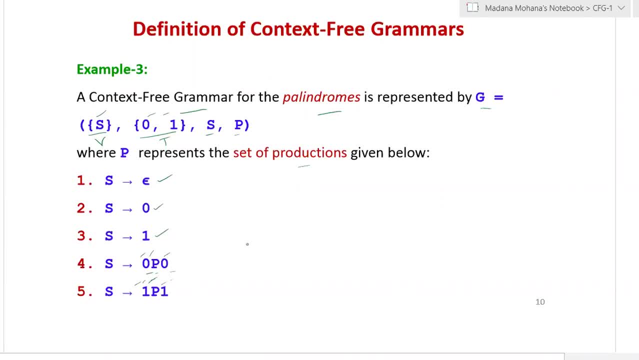 terminal. so whenever you can derive something from this grammar, always it derives palindrome strings. so now the restriction of cfg conditions. left hand side: you can see all productions started with a single variable. yes, same variable or different variable, but single variable should be occurred in any context grammar. right hand side: you can see either null or a terminal. 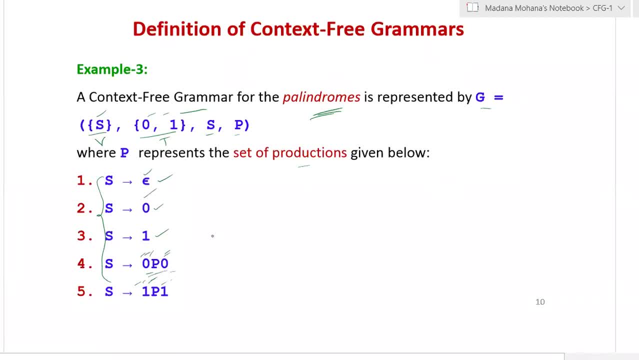 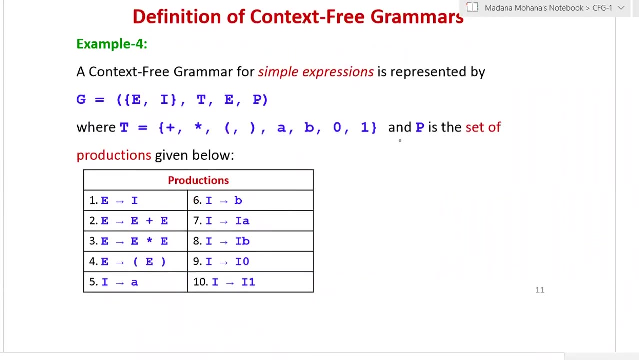 or string of terminals and variables, so it satisfies the condition of v union t whole closer. therefore, this is again a context free grammar. now another example. you can see a context free grammar for simple arithmetic expressions like calculator, represented by g equal to e comma i. so this set is called: 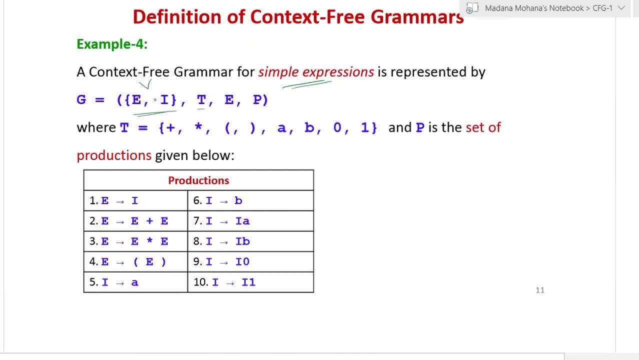 as v variables, then t, v, t terminals. then this is called as s. e is the start variable. now p is nothing but set of productions where terminals are given. below terminals are. see, this is simple expressions with consisting of digits, letters, arithmetic operators, parentheses, etc. now, place is automatic addition, star is automatic multiplication. then this is open. 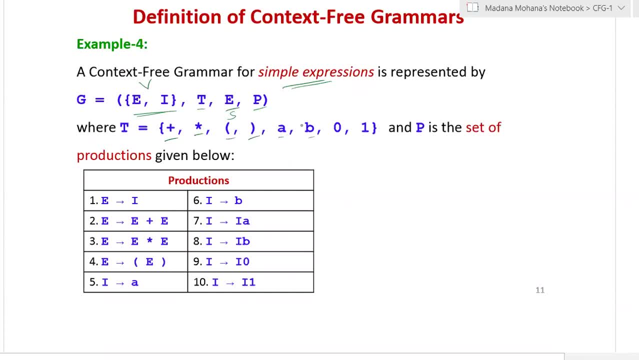 parentheses- closure. parentheses, then lowercase letter a, b or terminals, then digits 0, 1, also terminal. so these are all terminals, combination of all these terminals. the productions are given below table. now the first production: e derives i. he derives where he stands for expression, then i stands. 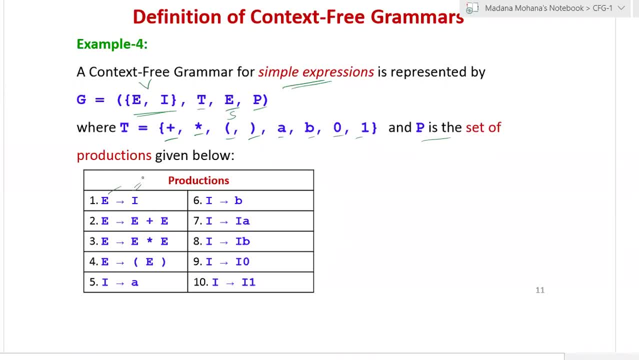 for value of that expression. so wherever uppercase letters, those are all variables. now e, defined as e, derives e plus e. this is arithmetic addition, expression plus expression, then e derives e into e expression, into expression multiplication, then e derives e within parallel expression, some values within parentheses, Then I, the I values are either terminal A or terminal. 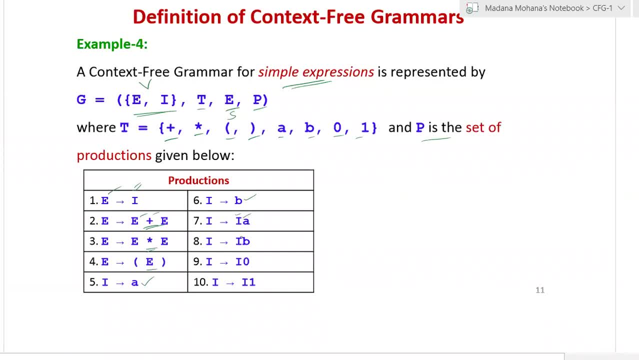 B, or I followed by terminal A, I followed by terminal B, then I followed by digit 0, then I followed by digit 1.. So these are all the various productions of the given grammar. So this grammar is also a context free grammar. The reason: left hand side it contains only. 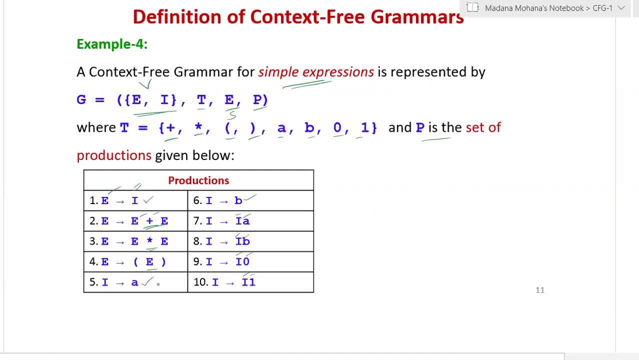 single variable- right hand side. it contains a single terminal or a single variable or variable, followed by terminals. that is string of terminals and variables or variables and terminals. So even null also allowed. but in this null is not there, Null is not mandatory, that is also allowed. So therefore this is again a context, free grammar. So this grammar: 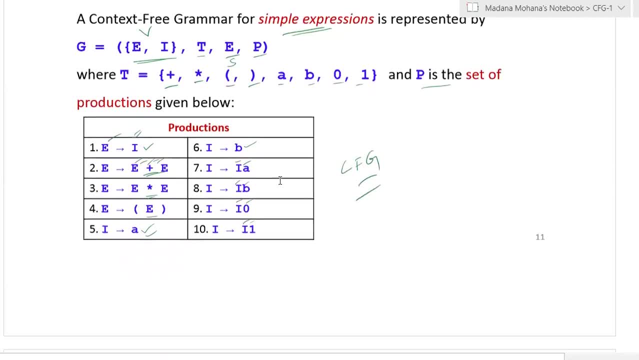 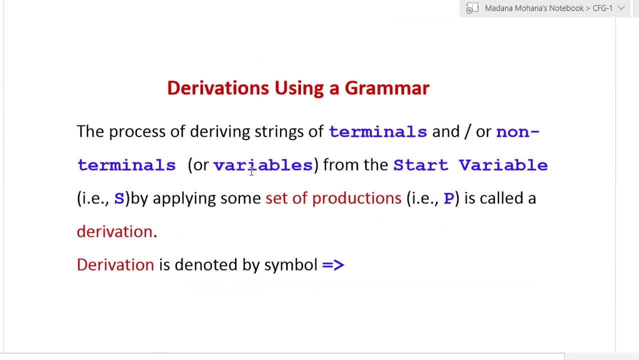 is frequently we will use for our problems This simple expression grammar. So that's all about a definition of a context, free grammar and various examples. Now we will move to next concept: derivations using a grammar. So first of all, what is the derivation? How? 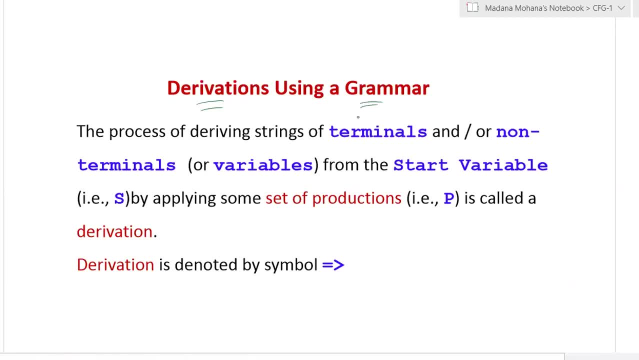 to find a derivation using our context free grammar. So coming to the definition of a derivation: The process of deriving string of terminals, String of terminals and or non-terminals, also called as variables from the start variable, that is, S In the grammar G, equal to VTSP, where S is start variable. How to derive strings. 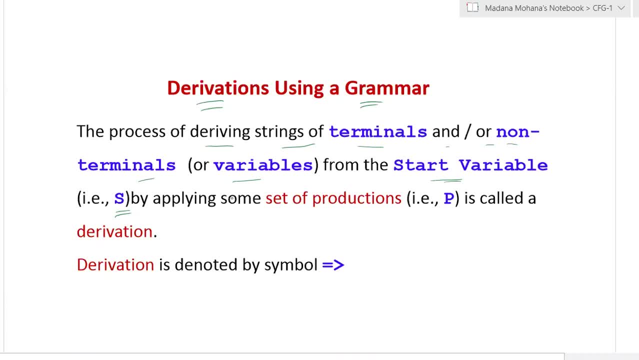 of terminals and or non-terminals from start variable, by applying some set of productions, By applying means, by substituting some set of productions from P. P is called a derivation. Derivation is denoted by a simple unidirectional double arrow. This we will call it as derives. 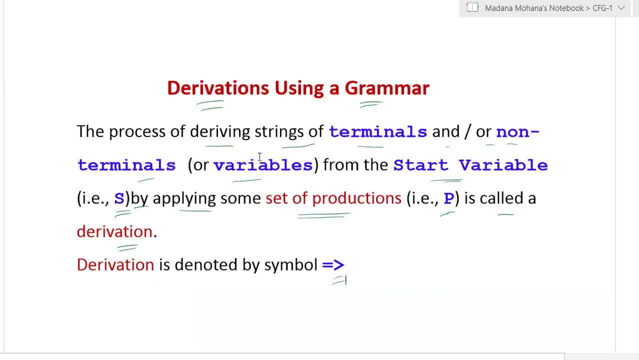 So this is the definition of derivation. So now from the given grammar, from the starting variable we can derive string of terminals or non-terminals, or combination of both the terminals and non-terminals, using start variable From the productions by substituting set of productions. that is called as derivation. 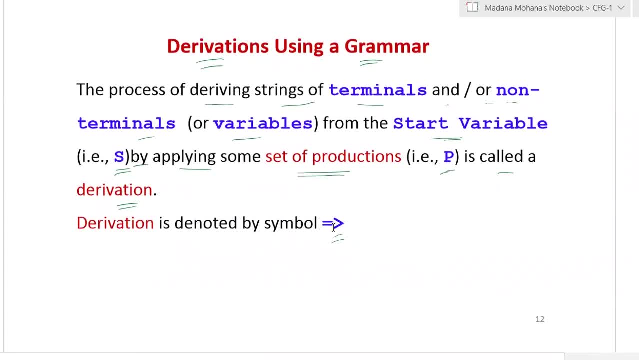 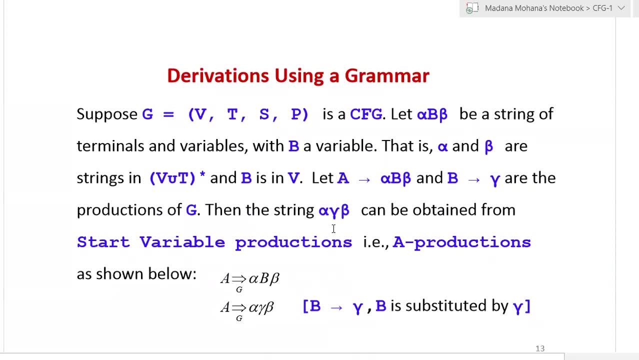 derivation is denoted by unidirectional arrow. so now see how to define a derivation formally. let us see a context free grammar: g equal to vtsv is a context free grammar. let a string- alpha, b, beta- be a string of terminals and variables. here in this, b is a variable. 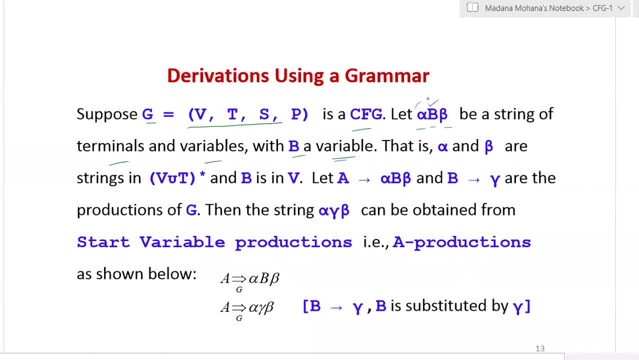 here b is a variable, whereas alpha and beta are strings. in v unity whole closure includes null, whereas b is in single variable from the set v. now let us take the productions: a derives alpha, b, beta is a production. a derives alpha, b, beta is a production and b derives gamma is another production. so these two are productions in the context. 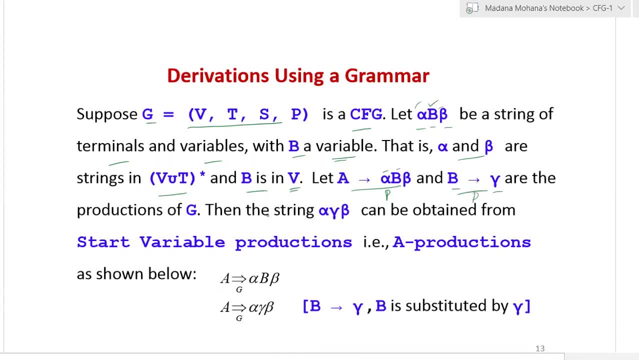 free grammar g. so now we have to obtain the string alpha gamma beta. how to obtain this string? our original string is alpha b- beta. now b contains a production. by substituting b value in this stringer. now b is replaced by gamma, then you will get a production of alpha gamma beta, and b derives. gamma is another production. so these: 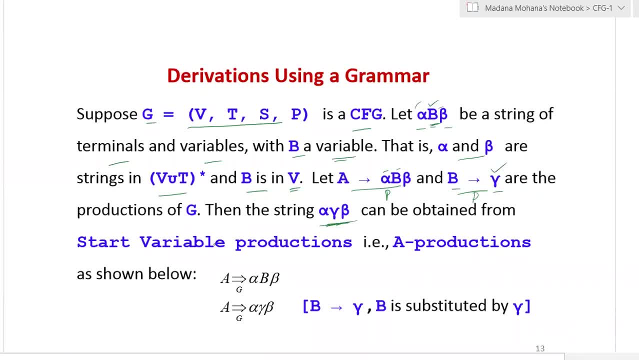 can be obtained from the start variable productions. so here the start variable is the by default. first production is start variable. so a derives alpha b beta. now take a derives alpha b beta in place of b in the right hand side of the production. substitute b derives gamma right. 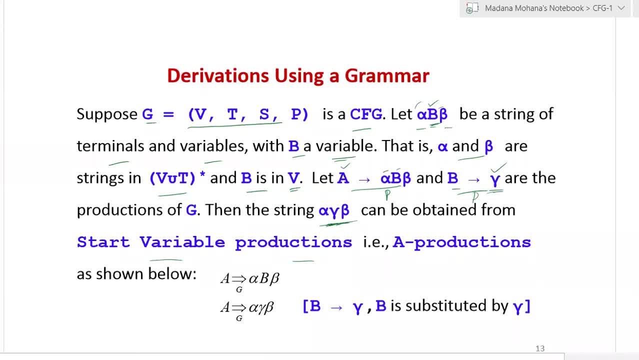 hand side value gamma. so then you can obtain alpha gamma, beta. so can be obtained from the start variable productions, that is a productions as shown below. so you can take the derivation like this a derives, so in normal production also. we will read it as the derives only, but 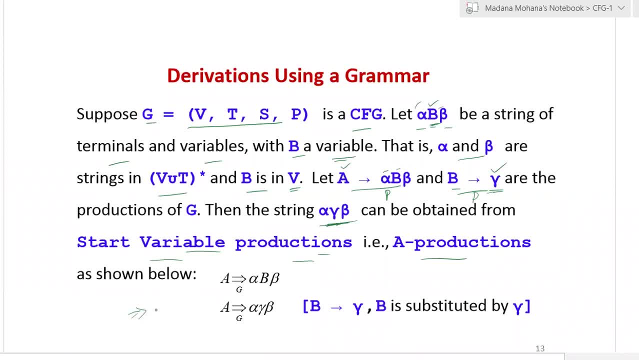 derivation will add double line unidirectional arrow. so now a derives. first you can take the starting variable, production. what is the production? alpha b beta. so a derives, alpha b beta. sometimes it is also called as equal a, equal to alpha b beta. so you can take the. 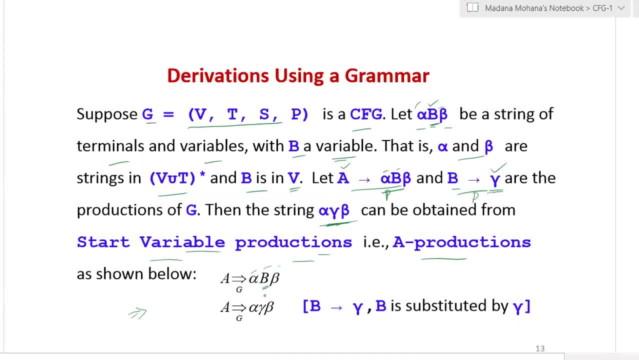 derivation of alpha and bigger than beta, which will be equal to alpha, where etaa is the derivation of alpha beta and therefore we have a better possible derivation so that the derivation is equal to alpha x, zeta, o, b, etaa. and also, when you take a derivation, 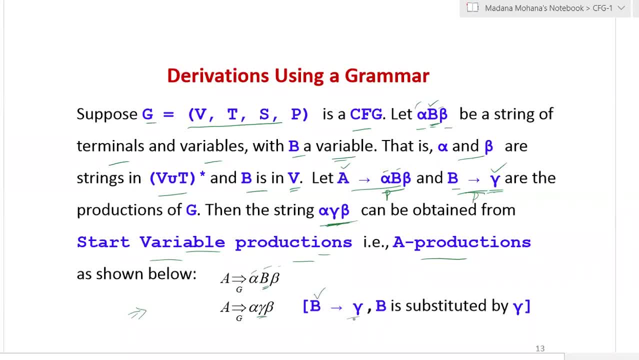 you get an equation like this where etaa is fa, e. so what we have- we can write an equation, name and a period of time, dear a brothy, which is v. this is n, equals to n is equal to 8, and now f is given as cent per day and v is joined with v dot 8. it is again from F for Desq dal. 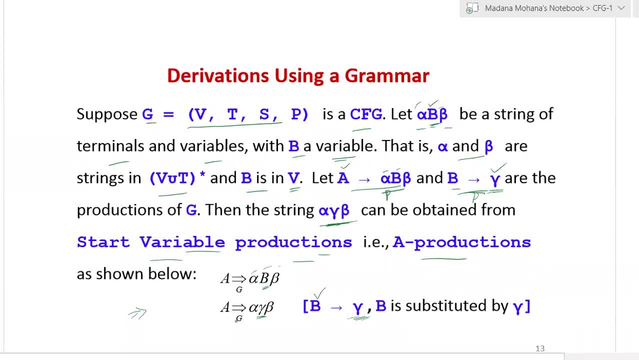 you can use the grammar name. g is the grammar for every step you can write on top. you can use so whether one step or two step derivation: that means only one substitution used or more than one substitution used. some notations are there that we will see, so this is called a derivation. 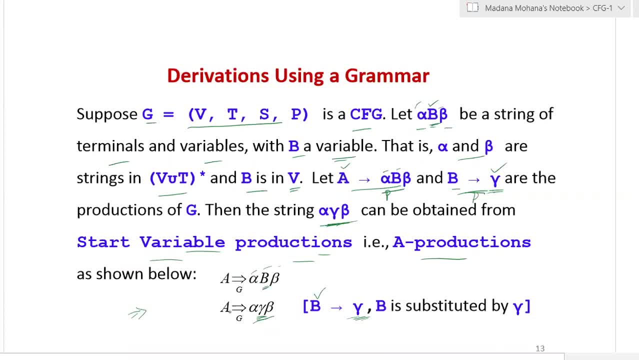 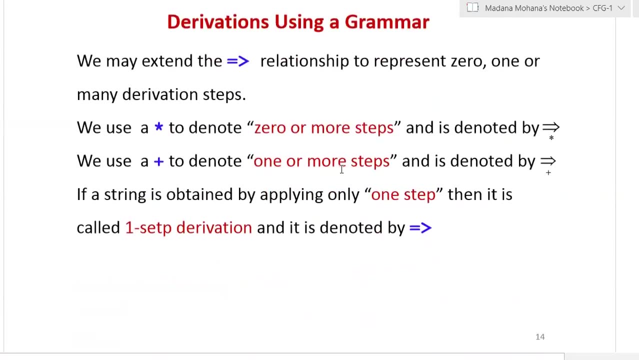 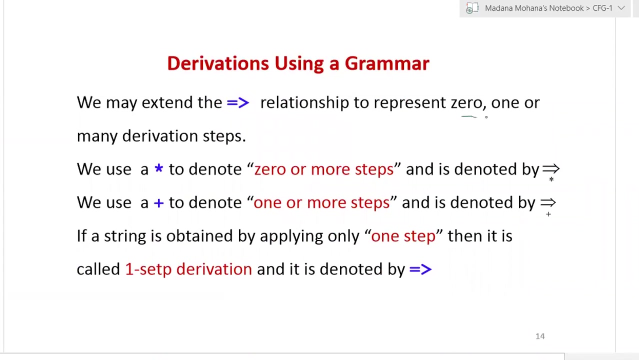 here who derived a string- alpha, gamma, beta- from the starting variable a by substituting the productions from the grammar, so this is called a derivation. now, here you can see. so we may extend the derivation, so this relationship to represent zero, one or many derivation steps. so zero steps. we did not apply any substitution, one step, we applied only one. 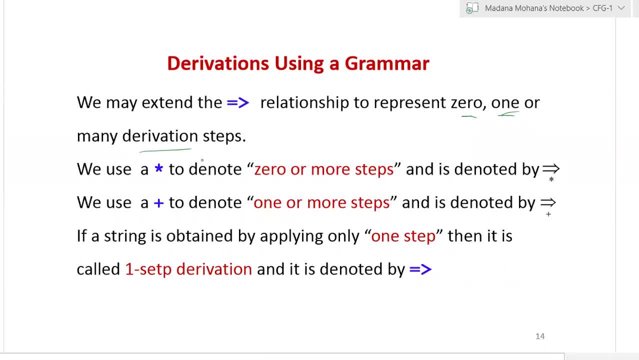 substitution, then many derivations. we applied more than one substitution, so for these we will use some notations. we use asterisk or star to denote zero or more. steps are used to derive a string, so and is denoted by so the arrow symbol bottom. we can use the asterisk. 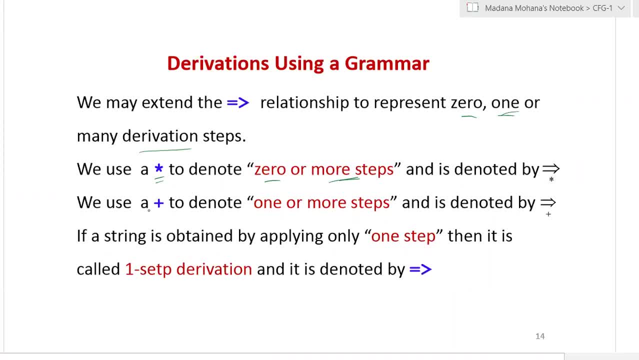 or sometimes we can use on top also. then we use place to denote minimum one, one step derivation or more steps and is denoted by with a positive closer, that is plus. if a string is obtained by applying only one step, then it is called as one step derivation and it is denoted by normal. 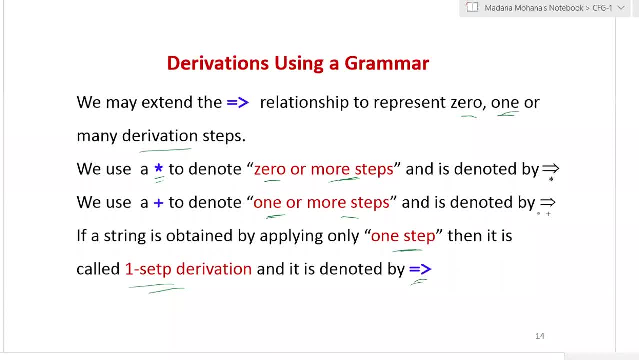 derivation symbol. so if we applied minimum one and more than one, we can use plus, then zero or more steps, then we can use asterisk only one step. we can use simply plus the arrow, without any asterisk, and positive closer. so these are all the notations we will use. 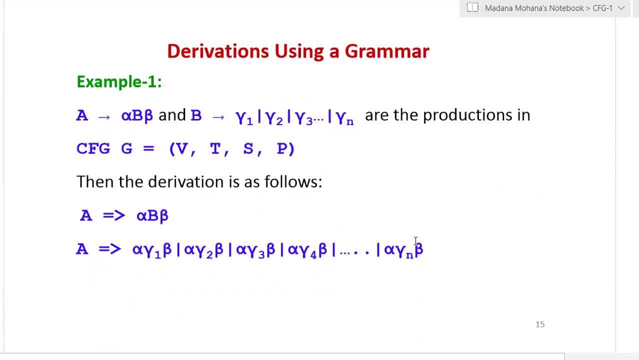 now let us see one example. so same example. whatever the example we discuss, that can be expanded with more substitutions. so we have a production: a derives alpha, b, beta and b derives gamma 1 or gamma 2 or gamma 3 and so on. gamma n are the productions in context, free grammar. 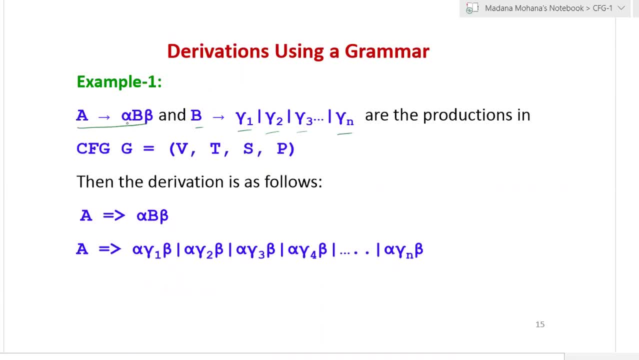 g equal to vt, a, s, v. now by default the first production left hand side variable, whatever. that is called a starting variable. so now the derivation can be obtained by taking the starting variable production only. therefore, first we can take starting variable a derives alpha, b, beta. so now in the right hand side. 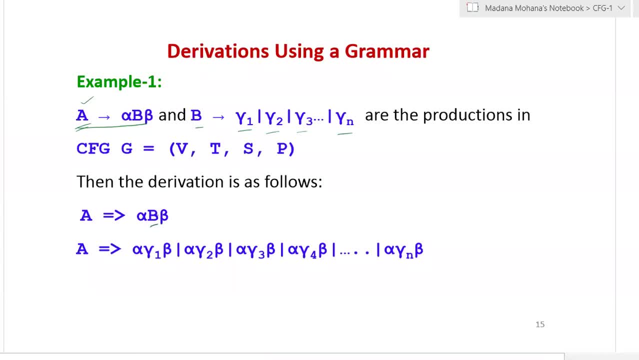 we have only the variable one, b, so b contains some productions, so you can substitute all these productions one by one. see how to substitute it: t and 10, and this can be written up the top. we can substitute all the number of time of this b, something called a straight. 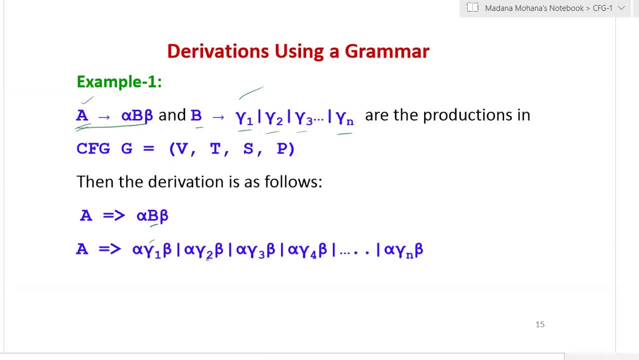 series and we can have a look at the pratic thing. so we can do this with alpha as alpha. alpha, alpha, and if we substitute this with alpha, gamma 2 are the morphological value, so company run: alpha, gamma 3, gamma 2, b, beta. then fourth value is gamma 4, so then and so on, n value, so gamma n. here you can see. 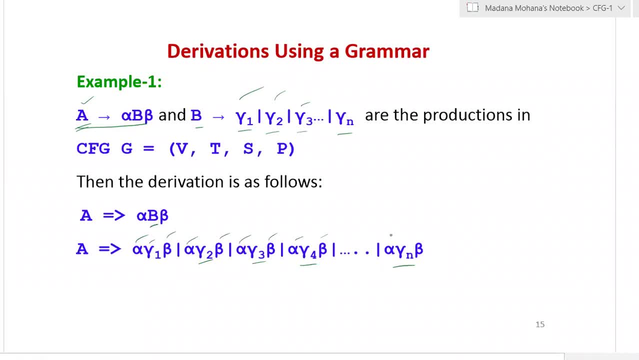 alpha beta are fixed for each and every substitution only. the varying value is b value. why? because b contains gamma 1 to n production, so n times you can apply the substitution. only one substitution you have to apply. so here we used to do: how many substitutions we use it, so we use it even zero. also, zero or more substitutions are. 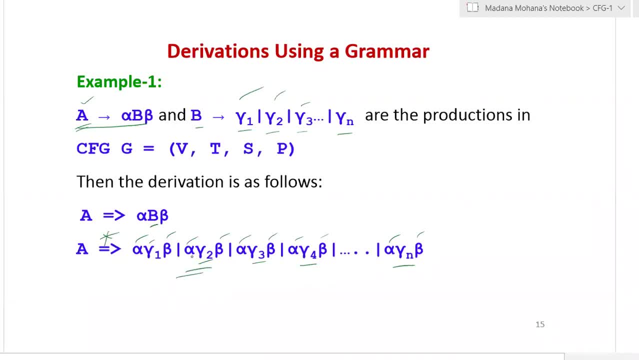 allowed here. so this is called as derivation here. what are the strings you derived? alpha gamma, 1, beta, 1 string. alpha gamma 2- beta is another string. alpha gamma 3, beta is another string, and so on. alpha, gamma n, beta. these are the strings derived from the gamma. 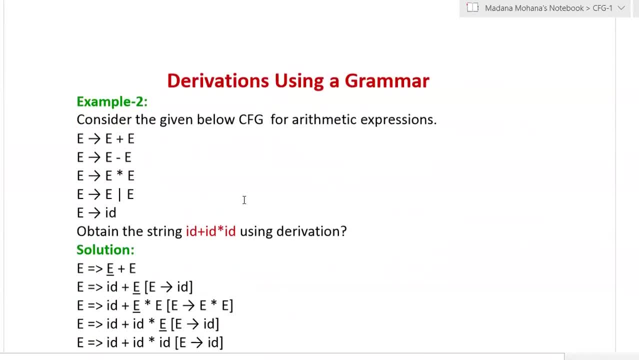 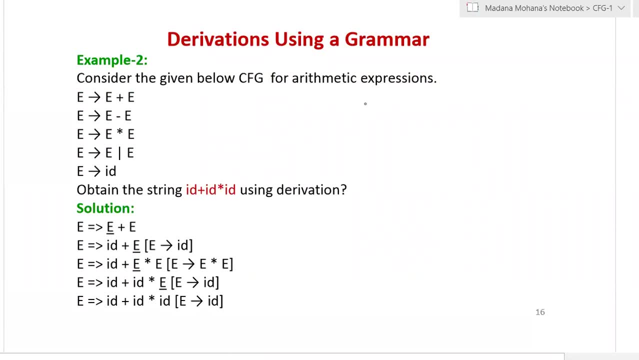 given grammar. so this is one example. see another example. so this is another important grammar arithmetic expression. so we saw one of the example, simple expression, grammar similar to that, this arithmetic expression. here it contains more automatic operations, so it contains addition, that is place, subtraction, minus, then multiplication, star, then division, divide, symbol, then id, here id. 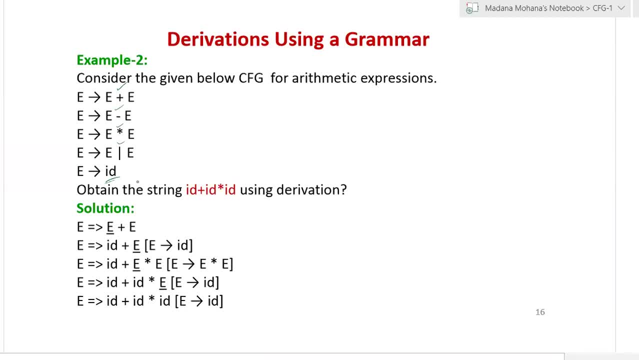 is a terminal. this will call it as a bold face string of terminal. but this can be treated as a single terminal, id. we can't treat id separately. so this is the special type of terminal. we will call it as bold face string string of terminal. so this is denoted by id, or sometimes. 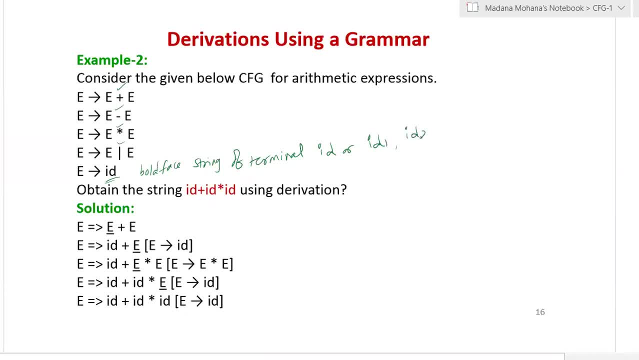 so i, i d one, id two and so on. so you can consider it as a single terminal, this one, wherever this will occur. now we have to obtain the string id plus id into id using the derivation, so we have to derive this thing from the given grammar. here you can see the given grammar, left hand side it. 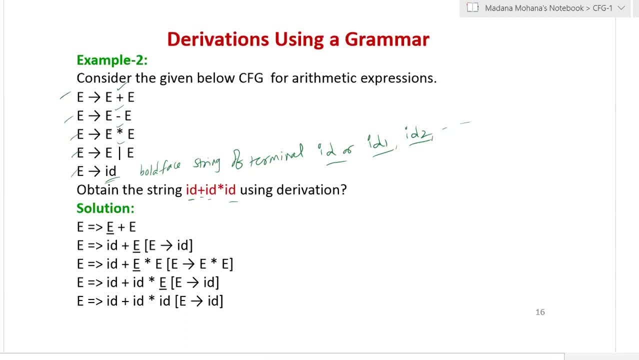 contains single variable, same variable it contains. so therefore e is called as a starting variable. you can see that it contains a single variable, so therefore e is called as a starting variable. so therefore e is called as a starting variable. you can take any production, but which production? 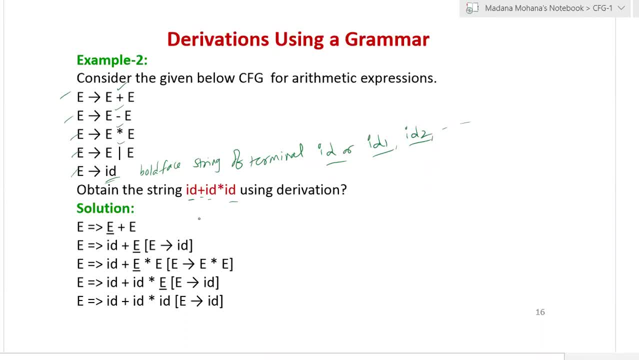 you need to take based on the string so needs to be derived for that which production is useful, for that only you have to take what it contains first plus combination, then into, so here place into combination. we have only the first production and third production, so those only you can take. 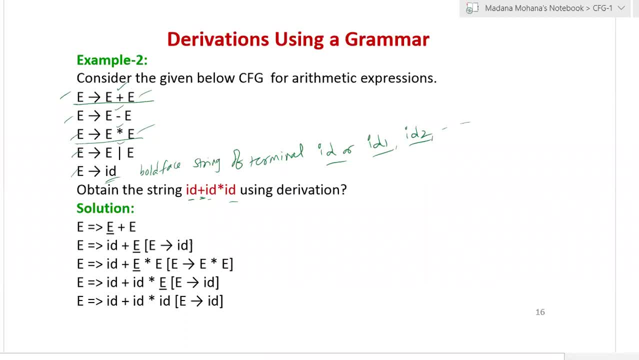 you can start with first production or third production. anyone you can take first. by taking first production, you can see by taking third also. i will explain here. so first take e, derives e plus e here what you have to do to derive the output string id plus id into id. so in place of variable in the right hand side you can substitute one substitution. 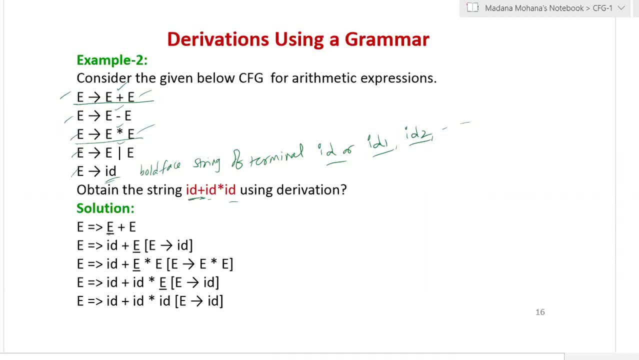 at a time. so the string must start with id. so left hand side variable e: that should be replaced by id only so directly we have id substitution for e. so you can substitute id here. now this will become id plus e. in bracket you can write down whatever. what is the substitution we used in. 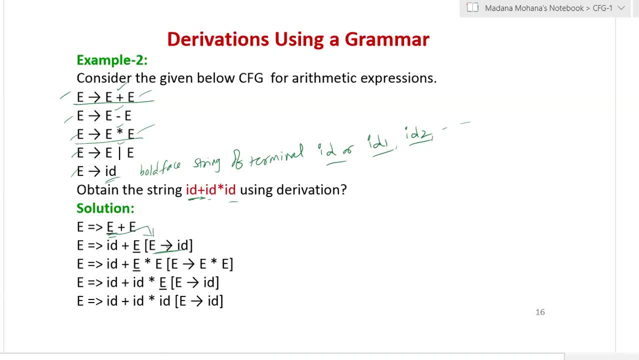 place of e. what you substitute: id. that substitution you can mention within square brackets in each and every step of derivation. now you can see id is derived, id plus plus already there. next third symbol: again what you want: id, but directly you can't substitute in place of id. why? because, again, 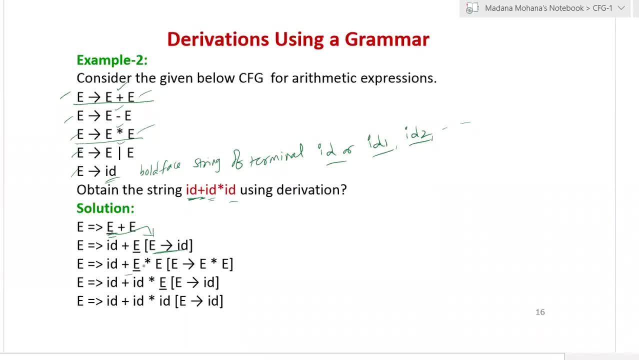 if you can substitute e by id. further, we can't expand a terminal, only variables are expanded. so now you can substitute. the remaining part is into, so into production. so in place of e we have e into e. so that is third production. e derives e into e. this 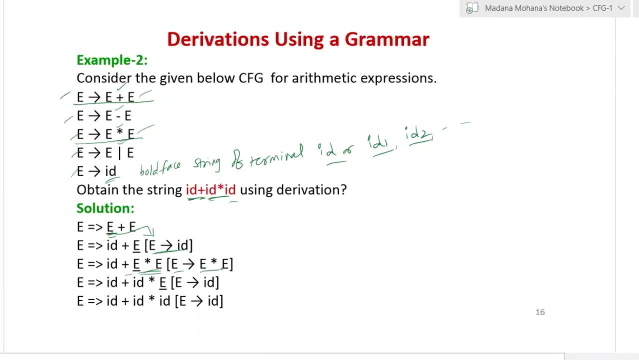 you can substitute here. so this is the substitution we use it. e derives e into e. now here, in place of variable, now you can substitute id directly. so now, what is the next symbol we want after plus? we want id. so therefore, in place of here- underline e- you can substitute id so that substitution of production listed here. so now id plus id into. 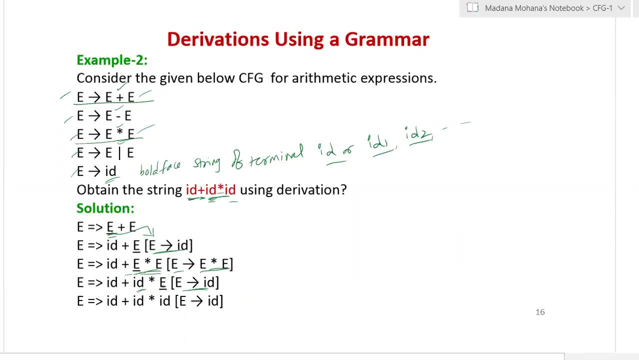 that is already there as thing. now last one: what you want again, you want id. so for e directly we have id substitution, so that underlined variable e you can substitute id. so now you will get id plus id into idc. this is our required string, so required string. so this is called. 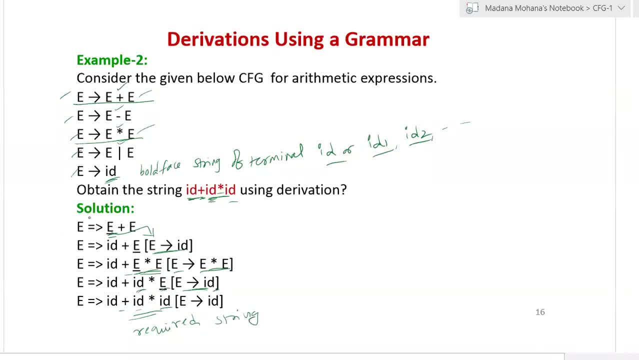 as derivation. so here you can mention: here we use zero or more productions are used, so use a stick, then bottom you can mention the grammar name also g. so it is not mandatorily. if you want you can mention. so this is called a derivation. so same derivation by taking third production at starting. 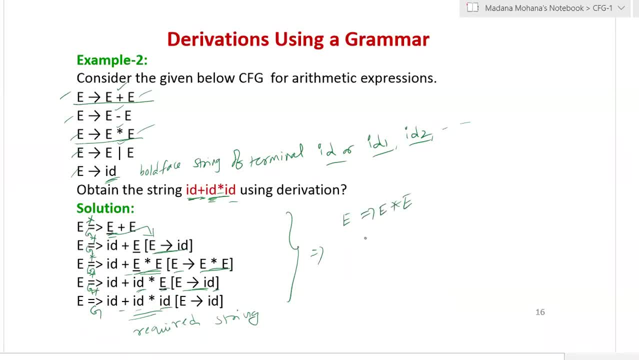 now e derives here. i will take e into g now. you can see now here: first what you want here into is there, but before into what you want plus. so leftmost e, you can substitute it by plus. so that is: e derives here. what is the substitution used? 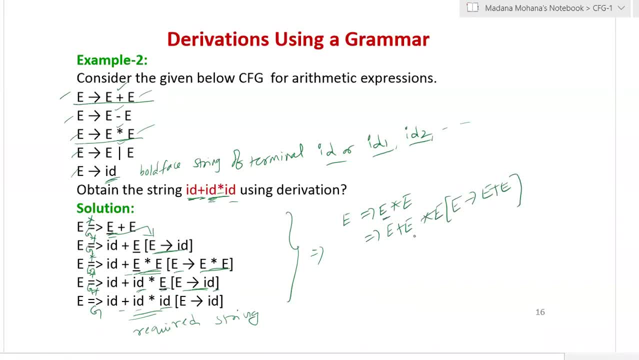 e derives e plus e. that is first. production is used in place of e. this is substituted. now this is in the form of e plus e into e. that means you can substitute id in place of e, id plus id into id. directly you will get but only one step. we have to apply each and every step of derivation. 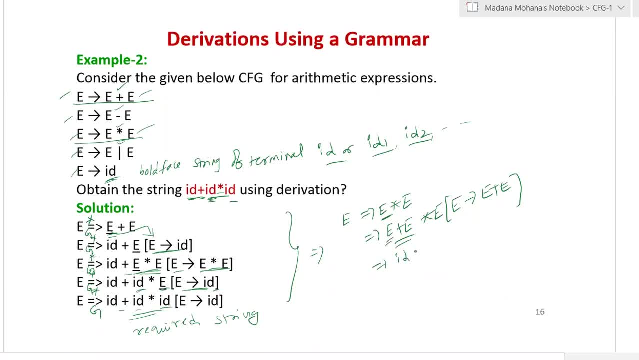 first leftmost e. you can substitute it as id. so id plus e into e. here what is the substitution we use? e derives id, so next e you can substitute again id, now id plus id into e. now remaining e is also there, so now that also you can substitute by. 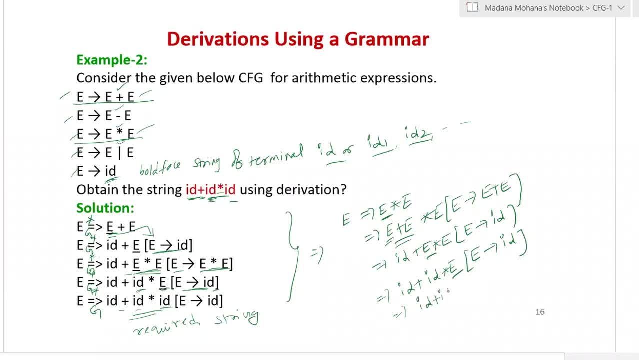 id. now this will becomes id plus id into id. now here what is the substitution we use? e derives id. now we can see our string is derived id plus id into id. so in both cases, by taking the first expression or third expression, so we derived our required same string. so 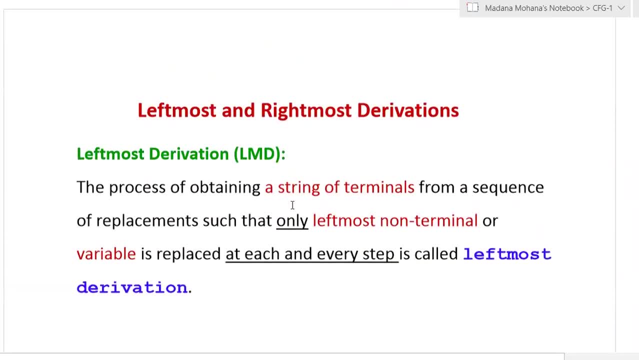 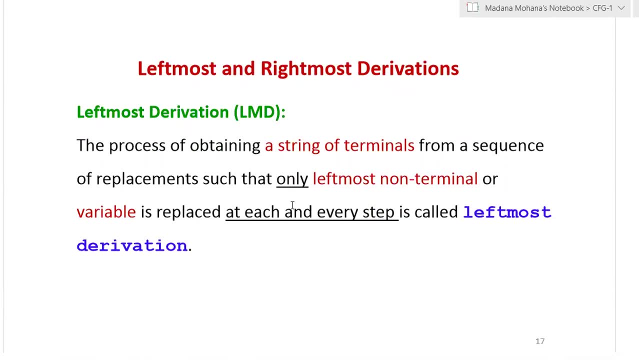 this is called as derivation. now we have various types of derivations, so the first type is called as leftmost derivation. so it is abbreviated as lmd is nothing but leftmost derivation. so how to define leftmost derivation? the process of obtaining a string of terminals. 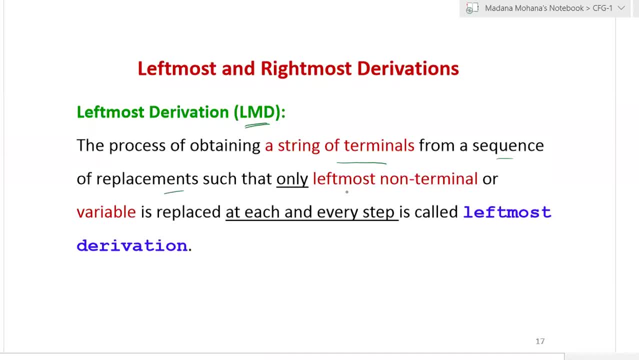 from a sequence of replacements such that only leftmost non-terminal or variable is replaced at each and every step of the derivation is called leftmost derivation. here you can see: leftmost derivation is nothing but same as the derivation, only the process of deriving a string in our previous example. whatever the method we followed, same process, but each and every step. 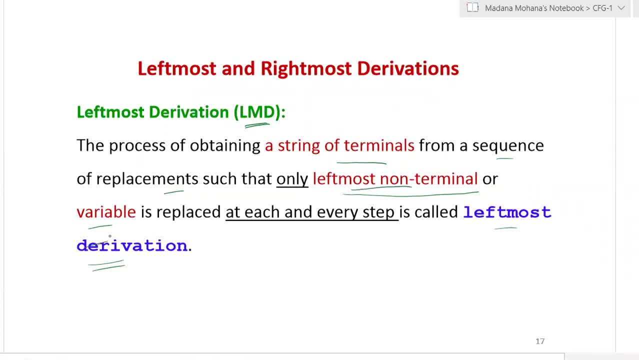 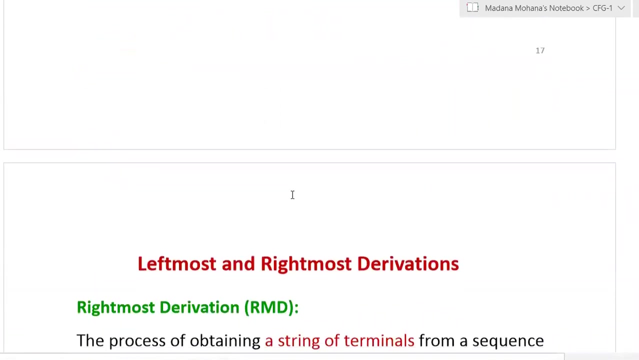 so only leftmost non-terminal or variable is replaced at each and every step is called as leftmost derivation. in our previous example we replaced sometimes leftmost variable, we replaced some sometimes rightmost variable. we replace it, but every step only leftmost variable is replaced. that is called as leftmost derivation, whereas another type we have. 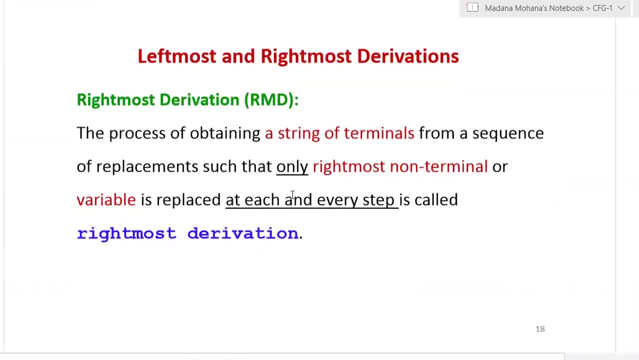 rightmost derivation also. so the rightmost derivation is nothing but each and every step of derivation. so we have to replace the rightmost variable. then there is called rightmost derivation- see the definition- the process of obtaining a string of terminals from a sequence of replacements such that only rightmost non-terminal or variable is replaced. 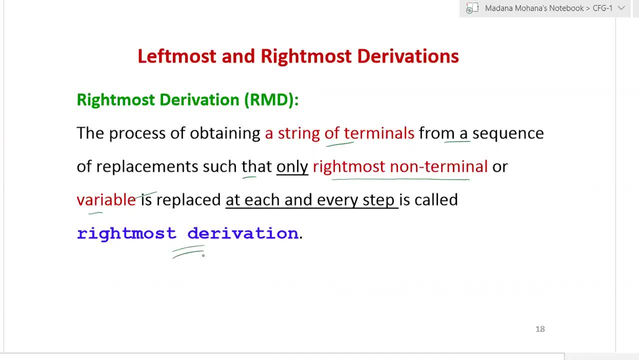 at each and every step is called as rightmost derivation. so each and every step, if you can replace a rightmost variable, then that is called as rightmost derivation in each and every step of derivation. so every time we can replace leftmost variable, then that is called as leftmost derivation. 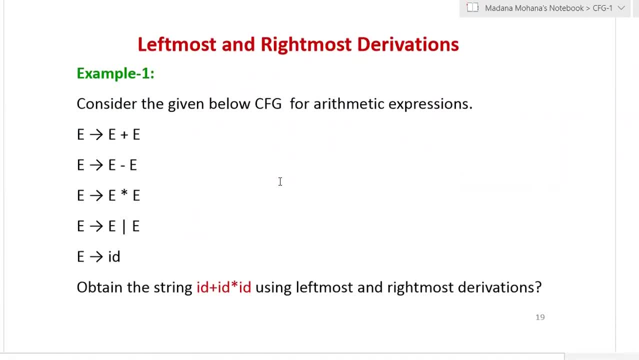 now we will see the same example. now we will discuss in terms of leftmost derivation and rightmost derivation. this is one important question in examination. so you will get a this type of questions: for the given context-free grammar, find leftmost derivation and rightmost derivation for the given string. so, like that, questions will be given. so now the question. 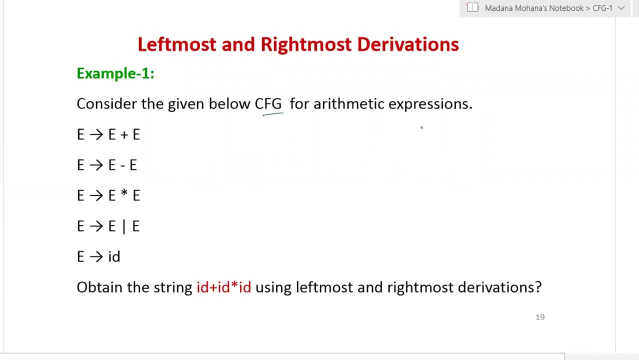 is: consider the given context-free grammar for arithmetic expression: same previous example. so e, ds e plus e, e, ds, e minus e, e, ds e into e, e, ds, e. by e, then e, ds, id now obtain the string. same string, what we discussed in our earlier example. 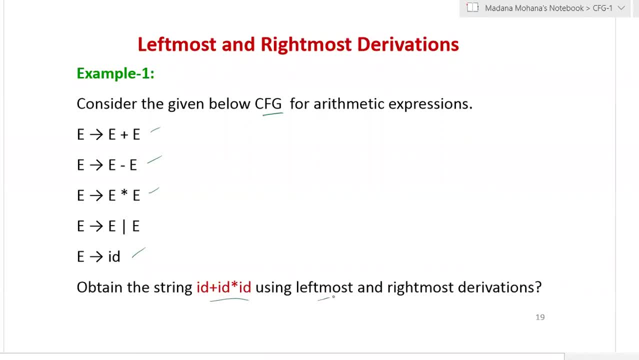 so id plus id into id using leftmost and rightmost derivation. already we have done one derivation, so in the similar fashion you can do, but each and every step you can replace leftmost variable and each and every step you can replace rightmost variable. then those derivations are called as: 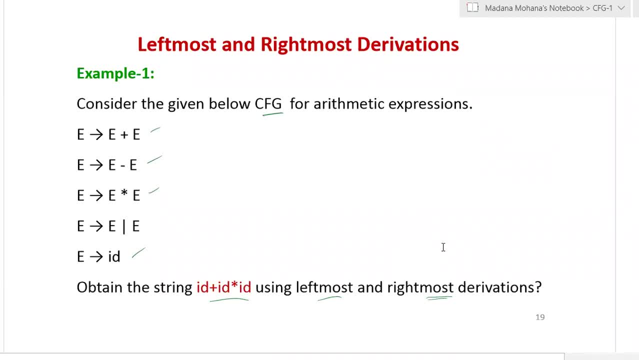 leftmost and rightmost, but you can't apply both leftmost and rightmost in one derivation. in any one derivation, every time you can replace the leftmost variable and instead of the rightmost you can replace only leftmost variable. leftmost to right side, left to right, whereas rightmost 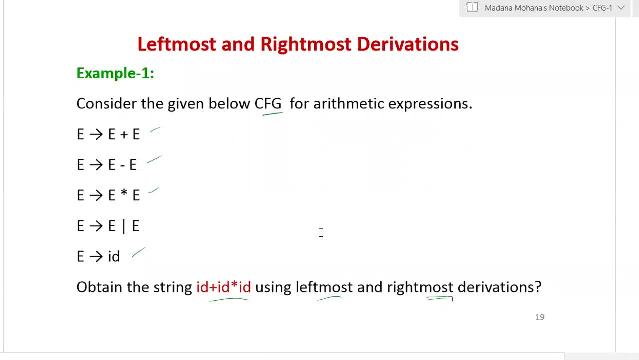 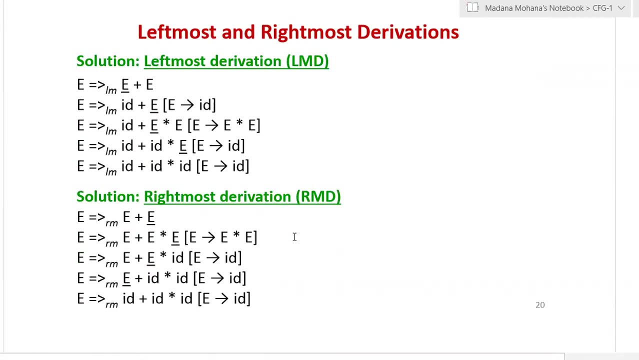 derivation or right to left side variable replacement. so in one derivation we can't apply both. so you can use either leftmost or rightmost at a time. now see the solution first. see the leftmost derivation. here also same. you can take either first two production or third production, no issues. but finally our required string needs to be derived. so 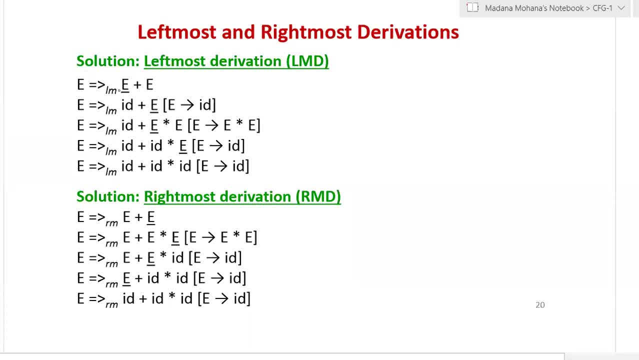 now leftmost derivation here first. so we have taken first two production: e derives e plus e. so the leftmost derivation you can replace, you can denote by suffix lm for our understanding, leftmost derivation. so e derives e plus e. here you can see we have two variables. so 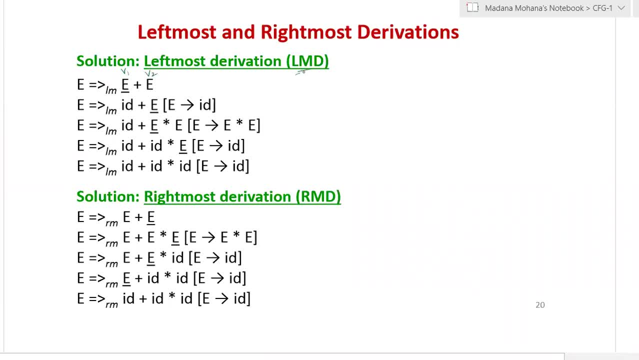 this is variable one, variable two. In case of leftmost derivation, what is the definition? each and every step of the derivation, leftmost variable is replaced first. so here two variables are there. first, leftmost variable, left side variable you need to replace so here. that is underlined here. so now in place. 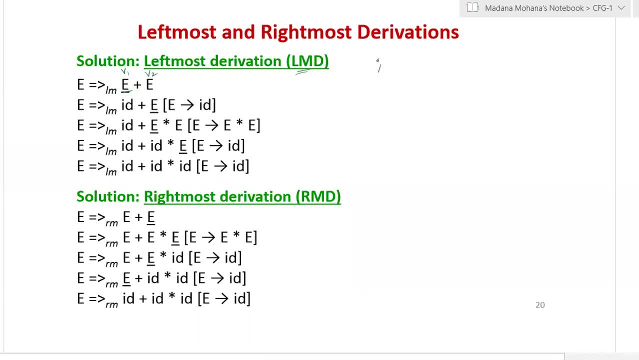 of e. what you need to substitute our string is here Id plus Id into Id. so our string must start with Id, leftmost. so leftmost what we have: E, e, p, g, e form. so first e is replaced by id. so this is replaced by id. now the substitution used here: 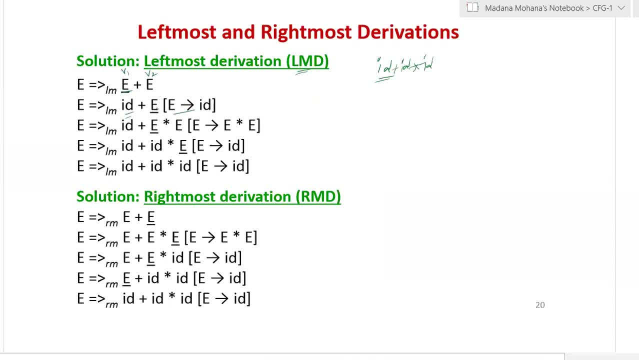 e derives id, now id plus e. here you can see only one variable. so either leftmost or rightmost, if we have single variable directly you can substitute. no issue. if more than one variable occurred in any derivation, always you can replace from left to right. so in leftmost derivation now you can. 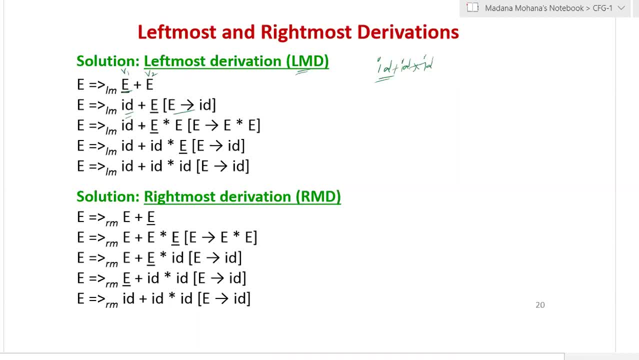 see here we have e, so id plus after plus what we want, id. but directly we can't take in place of e as id we have the expression into, so that into production you can take: now e derives, e is replaced by e, into e, so that is substituted here e into e again. you can see here two variables. 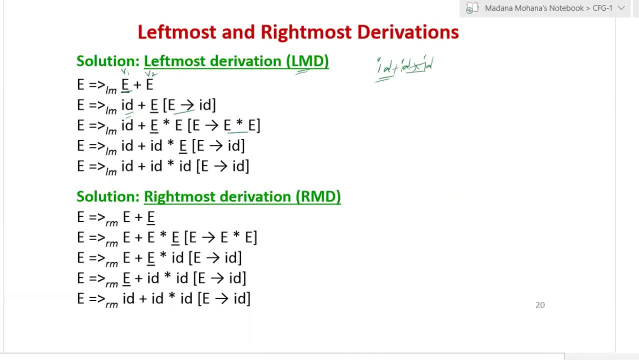 are there here. don't substitute rightmost e first. substitute leftmost here, so that e is underlined here. this you can substitute first. you can substitute leftmost here, so that e is underlined here, this you can substitute what you need to substitute here: id plus after plus what you want, id. so e derives, id now e. 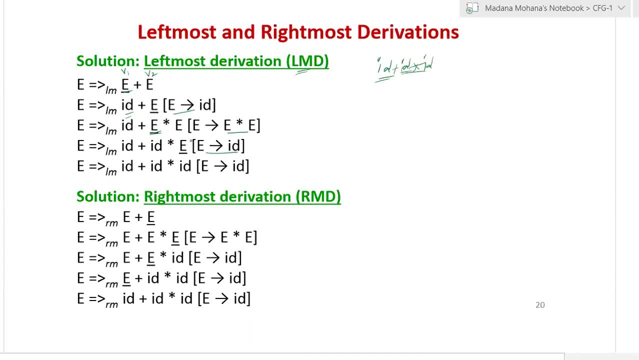 derives, id is substituted. then we have only one variable, either leftmost or rightmost. if single variable is there, you can substitute directly. if in case of more than one variable, then only you can follow left to right in case of leftmost derivation. now here g derives what you want now. 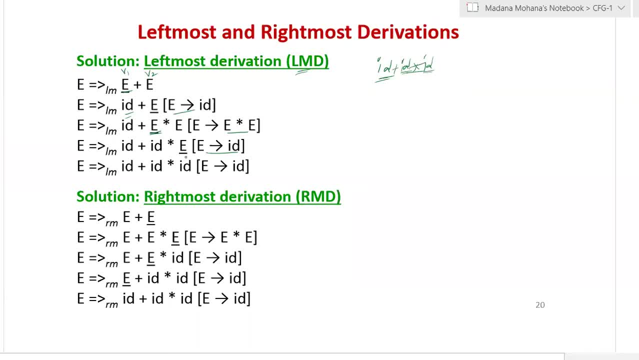 we got id plus id into. the last one is id. so in place of b substitute id, now e derives id. now we can say: this is our required string derived using leftmost derivation. each and every step we substituted the variables from left to right. similarly for rightmost derivation. you can see. 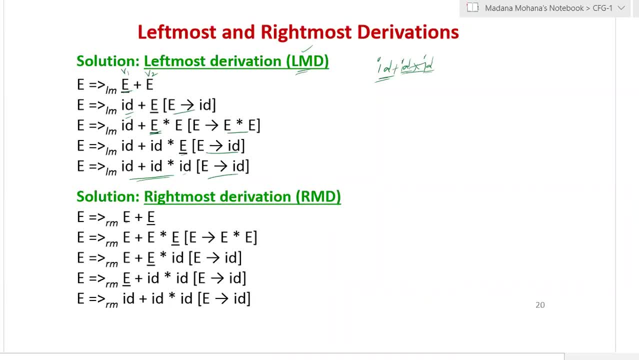 same process right to left: variable substitution, so rightmost derivation. you can denote rm, so under the derivation arrow. so now e derives e plus e. now two variables are there. first, we can substitute rightmost variable, so rightmost derivation. you can substitute rightmost variable, so rightmost variable. 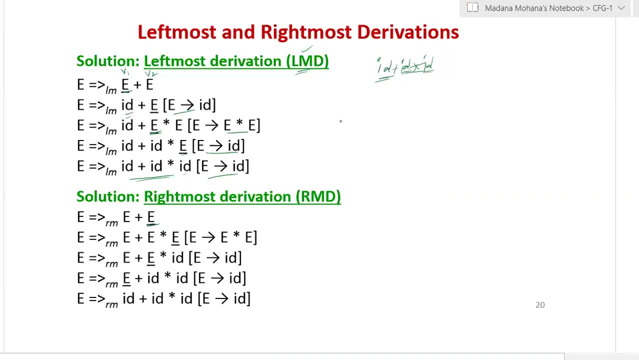 so rightmost after place, what you want see after plus, we want into. so rightmost e is replaced by into expression, so that is e derives e into e. now that is substituted here. now we can see, three variables are there in this step. rightmost variable first we can replace, so that is e. 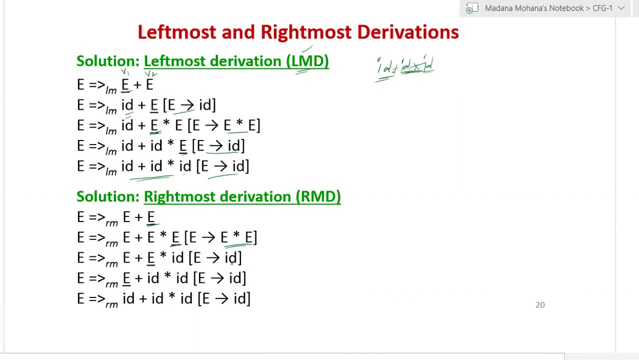 underlined so that e is replaced by id. so now, right to left, we are deriving this thing now, after substituting e by id, what you will get: e plus e into id, now id into before into so what you want: id. so now, here again, two variables are: 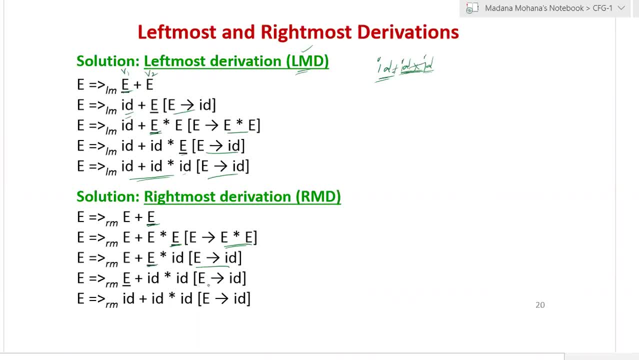 there. so rightmost variable is e. so this you can substitute by id. now e derives id. now you will get e plus id into id. now what you got here plus id into id, we got now what we want before, plus only id is required. now here you have only one variable, so here directly you can substitute the required. 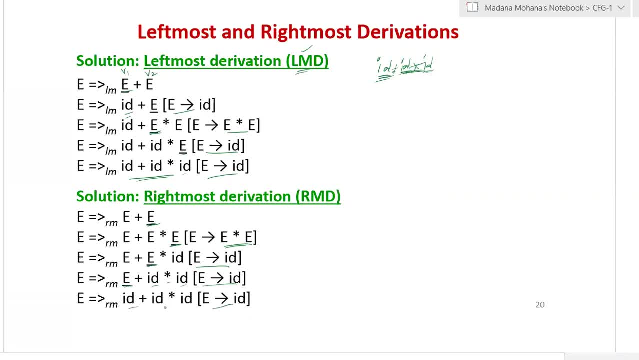 value, that is id, which is equal to half. so that s the actual step. we are stuck now here. we got id plus id into id 3, so we got the required string. now here you can observe either leftmost derivation, leftmost derivation, we got the same thing, rightmost derivation also. 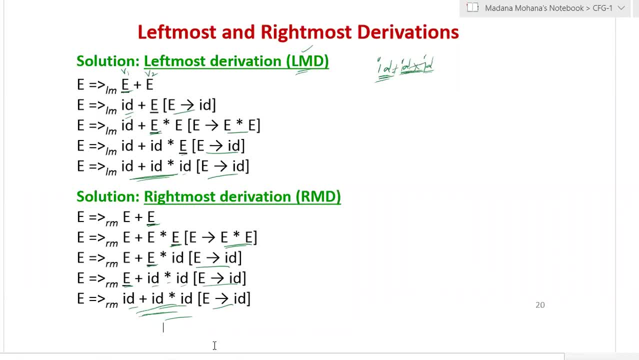 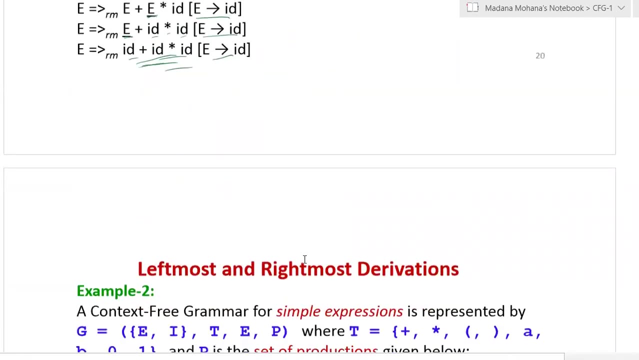 we got the same. so no problem, based on the concept for deriving either leftmost or rightmost, if you will derive same string, so that grammar is called as ambiguous grammar. that we will discuss later. that is our next topic. now let us see another example. so this example also we can. 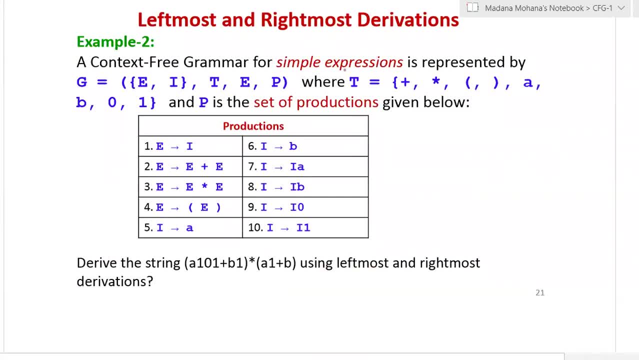 make it as practice also. so a contextual grammar for simple expression represented by g equal to this is v, variables e, comma, i now terminals. t, sc is e, now p, productions, where t equal to plus into open brace, closed brace, then terminal A, B, then digits 0,, 1.. These are all the terminals. The productions are this: 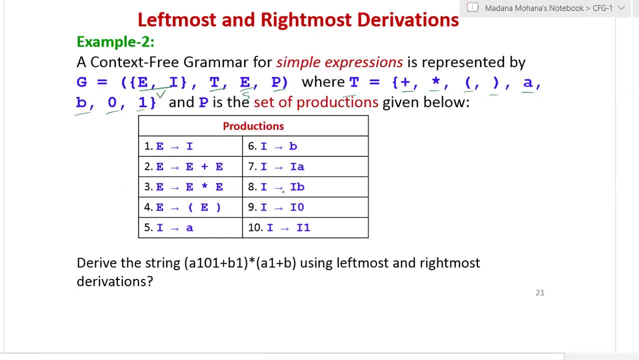 example we already seen in the contextual grammar examples. So these are the productions. Now we have to derive the string using leftmost and rightmost derivation. In the similar fashion. we can practice this problem. So the string is: open brace A: 1, 0, 1 plus B: 1,. closed brace. 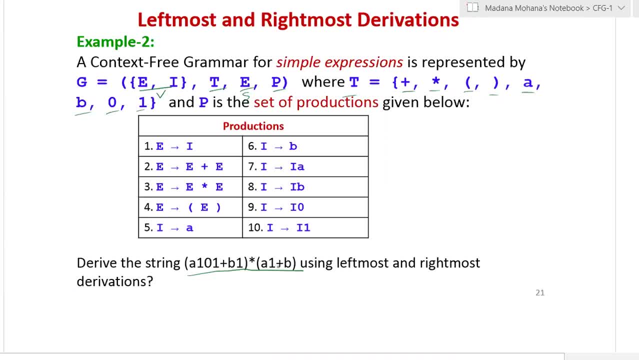 then asterisk again: open brace: A 1 plus B. closed brace. So you need to derive this string. So first leftmost derivation, you can take any production, then apply left to right variable replacement till deriving the required string, Whereas rightmost derivation take any suitable. 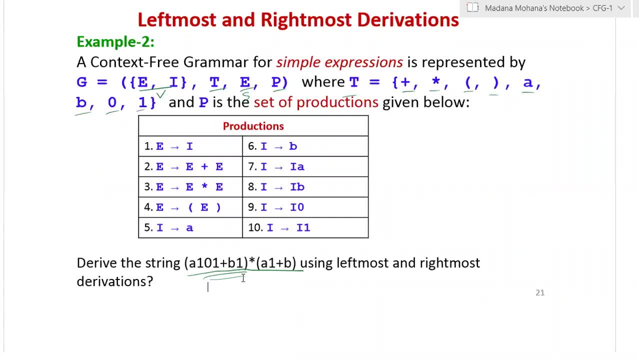 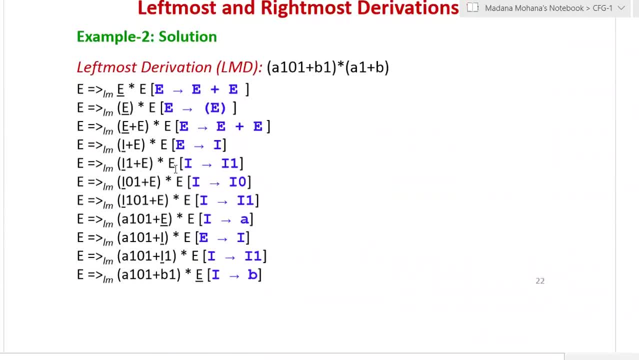 brackets, each and every step, you can derive the string. So, in brackets, each and every step, what is the production we use Here? I have provided solution also You can practice it. So if you have any queries, so you can post the queries, I will clarify. So the solution. 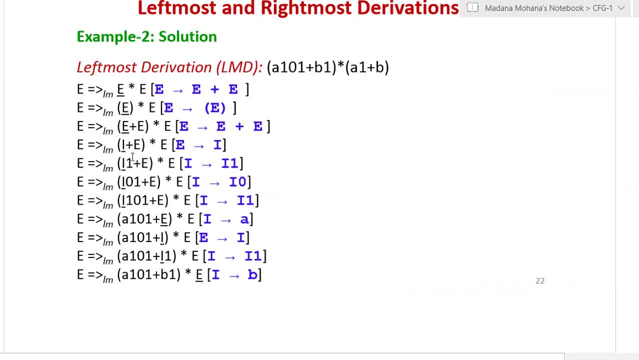 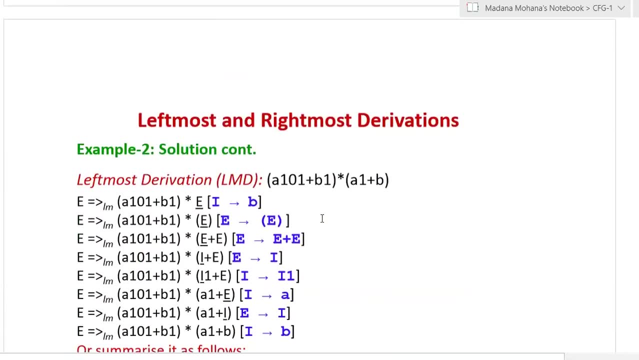 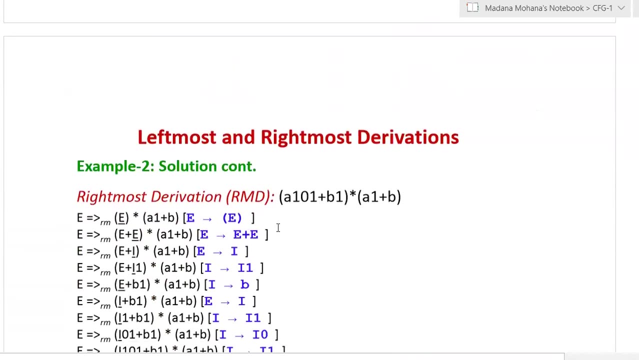 is already provided. So step by step, you can see how the substitution is used. leftmost derivation. Finally, you need to derive the required string Similarly for rightmost derivation so you can practice it. so like that you have to practice more problems, so that is called as. 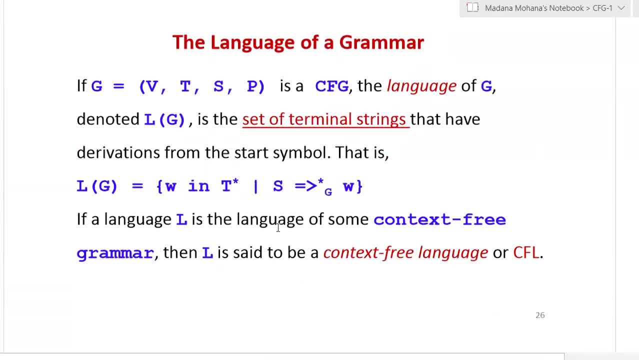 leftmost and rightmost derivations. then coming to next concept, the language of a grammar. so now we discussed about what is a context-free grammar, then how to define it, what are the various examples then? what is the derivation then? various types of derivations, that is leftmost and rightmost. 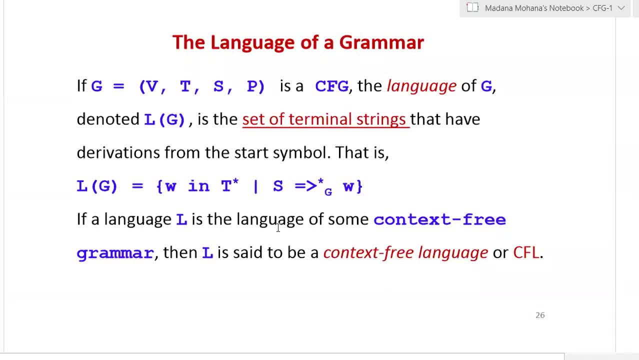 derivations. so now, how to define a language of a context-free grammar here. whatever the language we can define for a context-free grammar that is called as context-free language. that is, type two language. so how this can be defined: first, let us see a grammar g equal to vtsv. 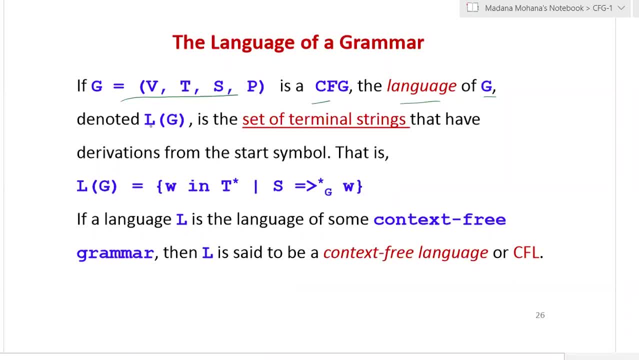 is a context-free grammar. the language of g is denoted by l of g is the set of terminal strings. the language is combination of set of terminal strings that have derivations from the start symbol. that is so. the language is defined by l of g equal to w. 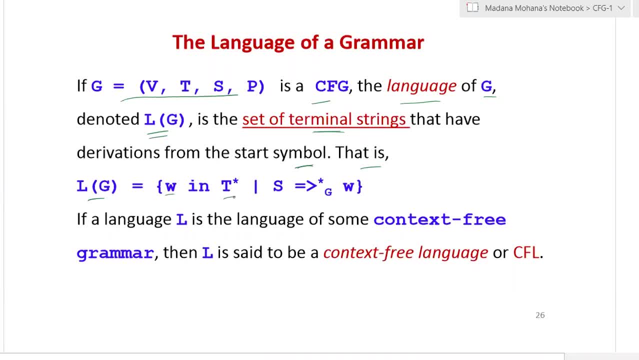 w is a string in strings of terminus that is t closer, such that so this w can be derived from the starting variable. starting variable is yes. yes derives w. here we used asterisk g. asterisk means zero or more. uh productions are used or steps are used, then g. g is the given context. programmer. 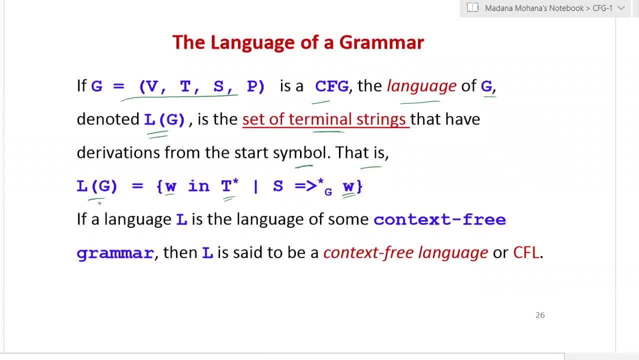 so from this you can derive a w. this is called as a long way. so if a language, l, is the language of some context-free grammar, then l is said to be a context-free language, or cfl so, which is type 2 language of chomsky hierarchy. so a language is nothing but string of. 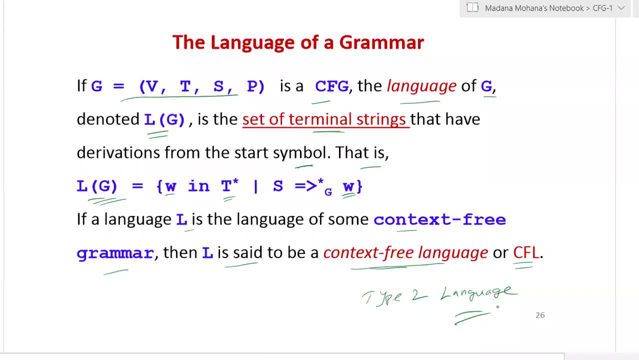 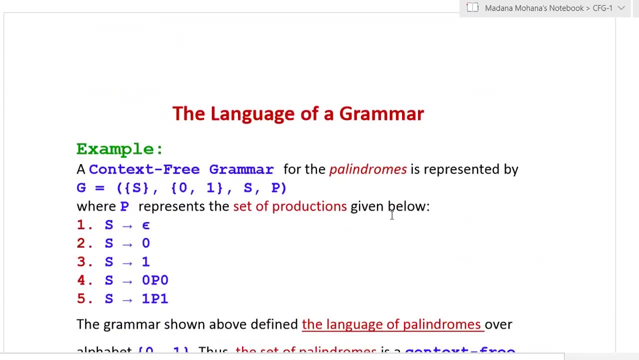 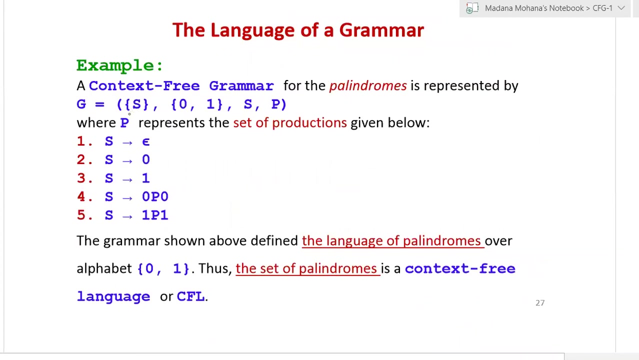 terminals so that have derivations from the start symbol. so this is the definition of a language. so how to define a language or a context-free language means. so this is the definition from context-free grammar. now let us see one example. a context-free grammar for the palindrome is represented by g equal to s, that is a variable v, then 0 comma 1. 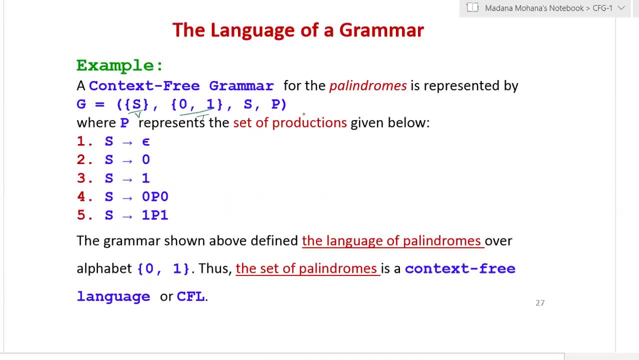 are terminals, then s, p, then p is represents the set of production elements are given below. so s derives epsilon, s derives terminal 0, s derives terminal 1, s derives 0, p, 0, that is terminal, variable terminal. then s derives terminal 1, variable p, terminal 1. this is: 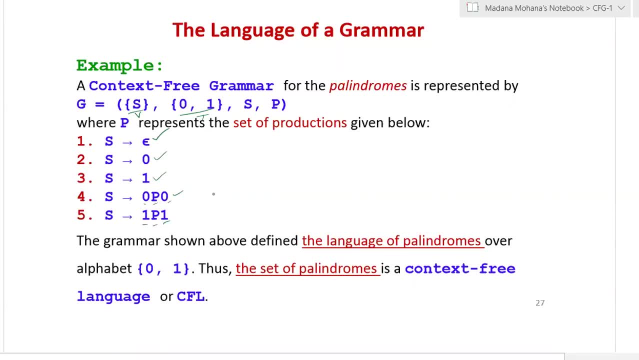 palindrome context-free grammar. this example also we discussed earlier now from this. so how to define the context-free language? the grammar shown above defined the language of palindromes over alphabets 0 comma 1. thus the set of palindromes is a context-free language or cfl. so like that we. 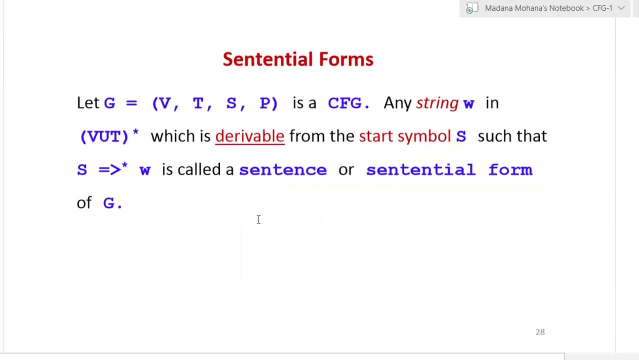 have to define. then, coming to next concept: sentential form. so what is the sentential form? this sentential form is somewhat similar to derivation, but see how to define this one. let g equal to vtsp be a context-free grammar. any string w in v unity whole closer. 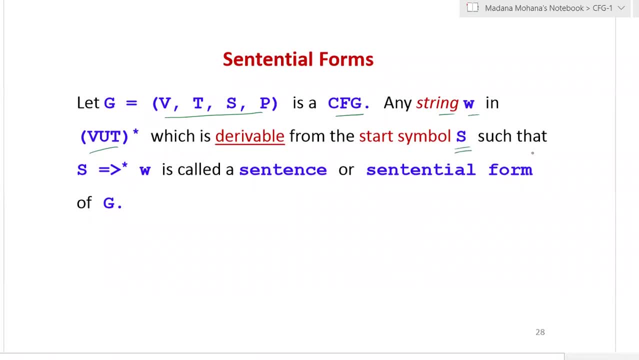 which is derivable from the start symbol here, such that s derives under asterisk w, is called a sentence or sentential form of g, so which is called as derivation, same as derivation here also from start symbol. yes, we have to derive a string, w- but where that string can be derived, the string can be derived from variables or terminals, or string of a string's text used mixed werden. we have to if we have to describe the string as such, which is called derivable from the start symbol s, with here also from start symbol as such, that we have to derive A string W. Но The string Can be derived. The string Can Be Derived From Verbal, An Lau果 To Tree AND powers, Which is derivative ofesta string W. But there are various terms and terms ofー. oh, you can be derived from variables or terminals or string ingredients of a string Of The strings. When can be derived from Didn and be derived from styles or termin- I don't have both existing whose, which is derivative from variousênз. We have to. 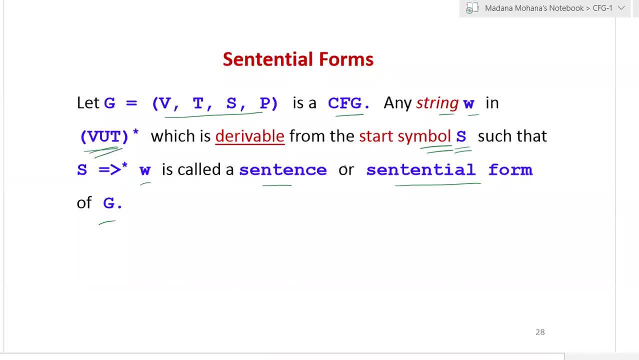 variables and terminals, including null. so that is called as sentence or sentential form. now in our derivation each step, whatever the substitution we applied, that is also called as a syntax. so then each step we have sentence or sentential form. here also we have two types of sentential. 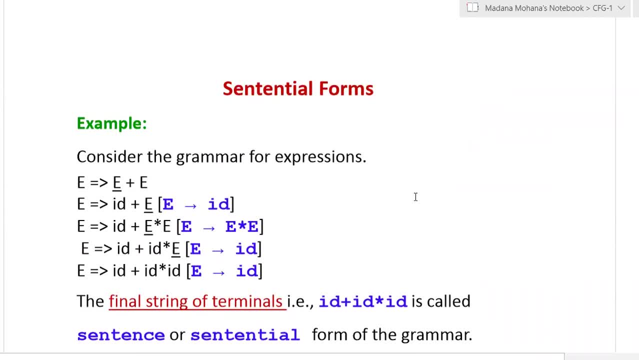 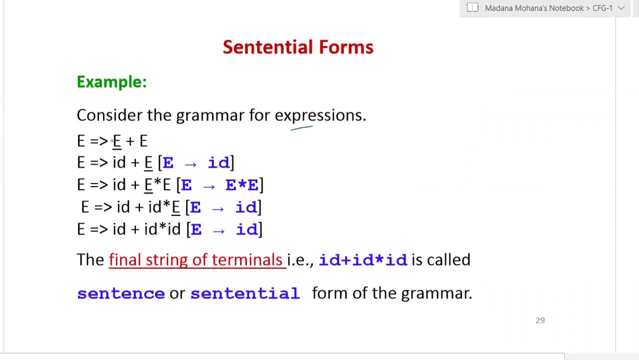 forms same as leftmost and rightmost derivations before that. so let us see example of sentential form. so consider the grammar for expression: same grammar. so now e derives e plus e. here you can see we used again the derivation concept leftmost e. now we substituted id id plus e. 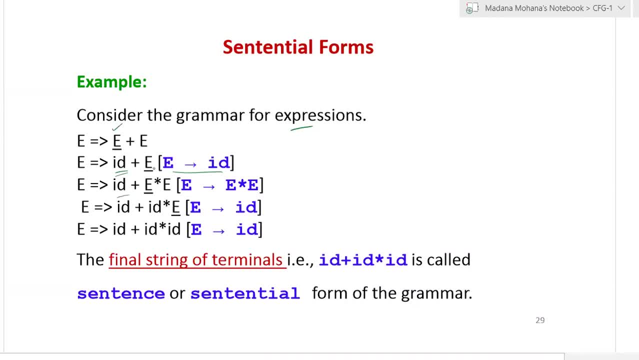 now e derives id. this is the substitution. then id plus. now next e is replaced by e into e. that is e, d, e into e. so then again leftmost e. we substituted id. so now here e d s id. now next we have one more e, that is also substituted by id. now we will get id plus id into id. here you can see: 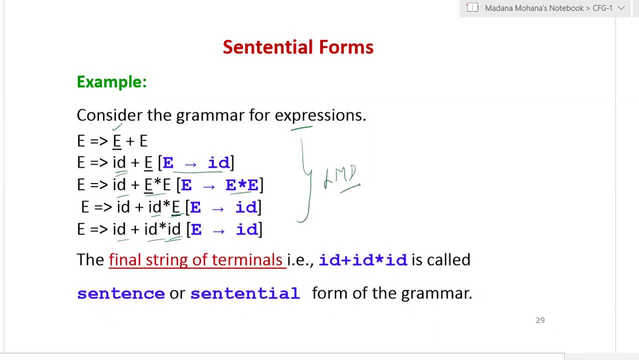 we applied here leftmost derivation. each and every step left most variable is substituted. now you can see- here we are talking about sentential form- from this derivation, how to define a sentential form. the final string of terminals, that is id plus id into id is called. 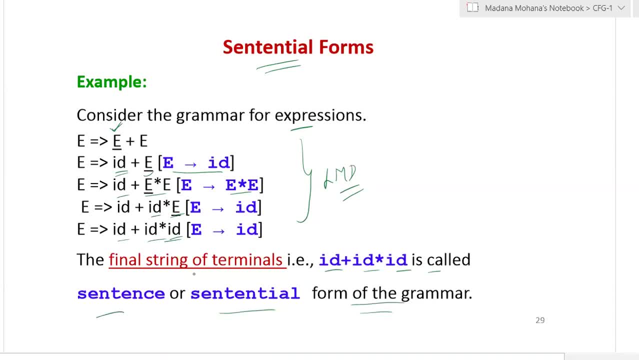 a sentence or sentential form of the grammar, so this is called as sentence or sentential form. then each and every step also suppose, if you will stop here, this is called a sentence or sentential form. if you will stop here, this is called a sentence or sentential form, if you will. 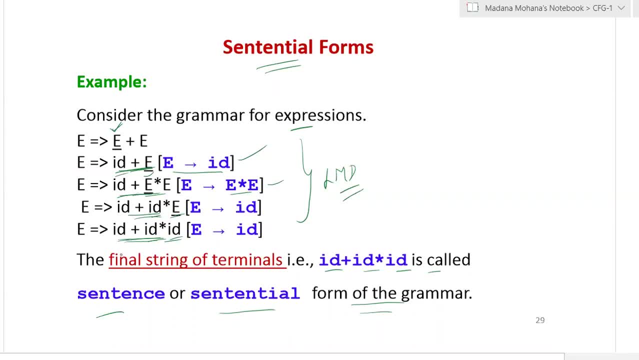 stop here. this will call it a sentence or sentential form, like that at the end of the derivation. the last one will call it as the final sentence or sentential form of the grammar. here also, you can see, here also we have a sentence or sentential form of the grammar, so this is called. 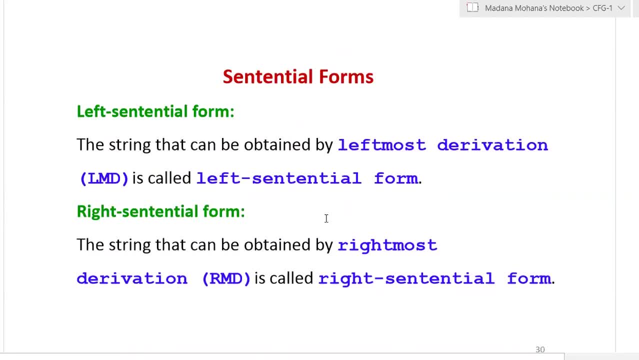 we have two types of sentential forms. so one is left sentential form, so another one is right sentential form. a sentence that can be derived using leftmost derivation is called as left sentential form. so a string that can be obtained by rightmost derivation is called as right. 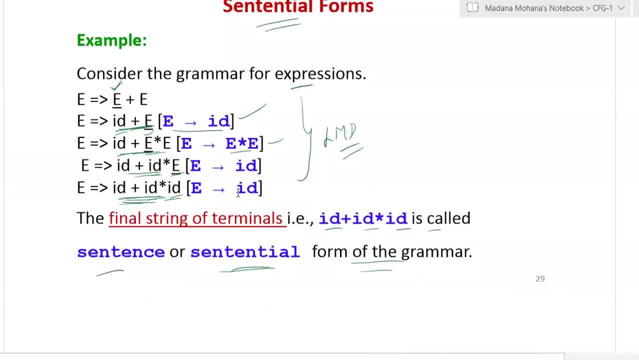 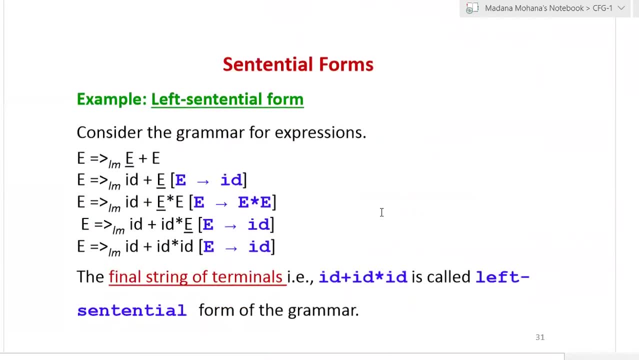 sentential form. so now previous example: here we use leftmost derivation, so here, whatever the sentence we obtained, that is called as left sentential form. then, by the way, we have by using rightmost derivation. so whatever the sentence we will obtain, that is called as right. 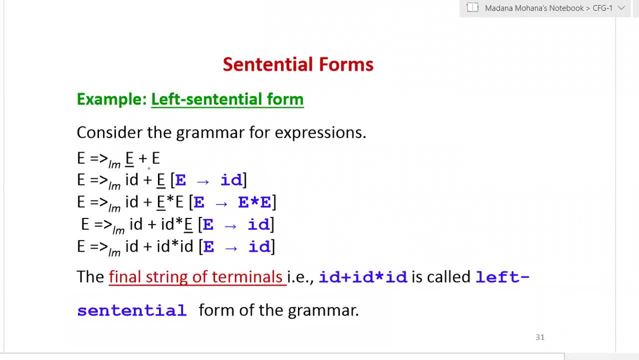 sentential form. again same example you can recall. so here you can see what is the derivation: here we used leftmost derivation. so using leftmost derivation, so here we derived the final string, id plus id, into id. so the final string of terminals, that is id plus id into id, is called as. 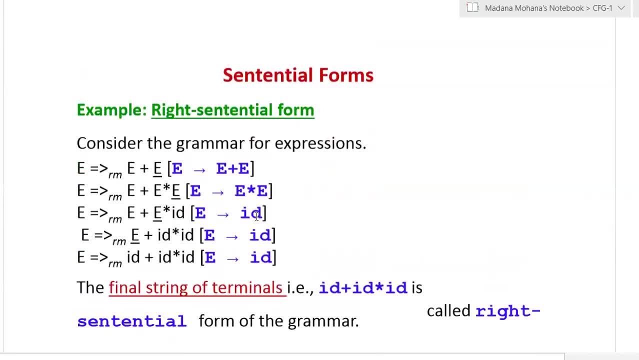 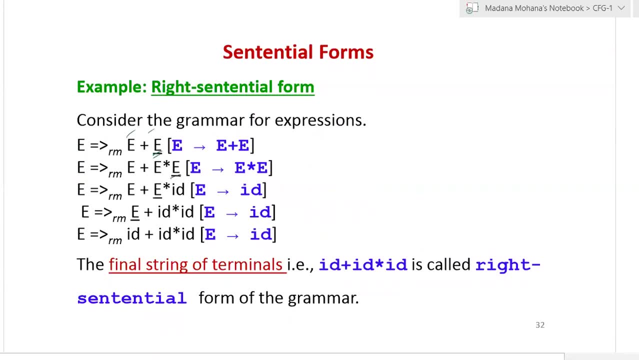 left sentential form of the grammar, similarly rightmost derivation. now here you can see that you can see here two variables: rightmost variable is substituted in three variables. rightmost variable is substituted, so now this is called as rightmost derivation. so here you can see the final string, id plus id into id. the final string of terminals, id plus id into id, is: 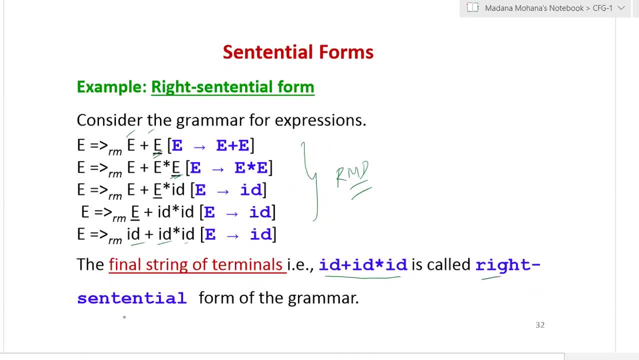 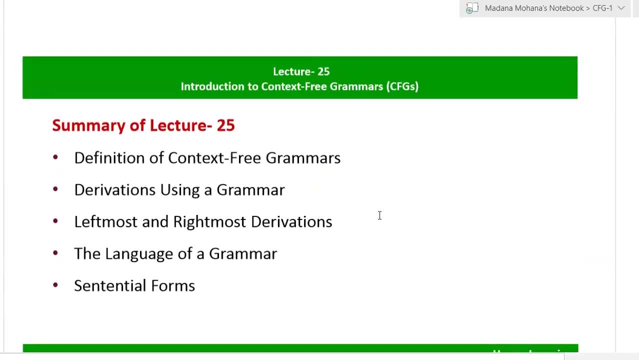 obtained by using at most deviation, so which is called it right sentential form of the gram. so these are all the two types of sentential forms, left to sentential form, on right sentential form. so now we stop here. then see the conclusion. so what we discussed in this lecture, first we 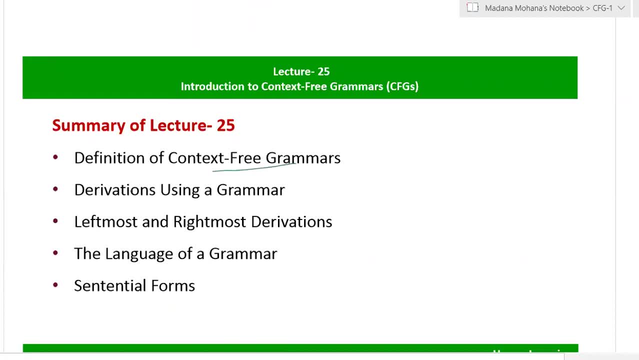 discussed about definition of context free grammar, followed by examples, then derivations using a grammar, followed by examples, then two types of derivations we discussed, that is, the leftmost and rightmost derivation, followed by examples, then the language of a grammar, how this can be defined. that language is called as context free language from the grammar g. then, finally, we discussed about